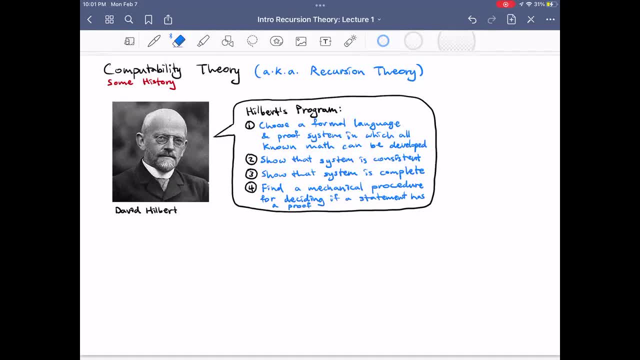 I'll skip some details, but I'll try to give enough details to actually give a real sense of why things work. So I wanted to start with just some comments on what the historical motivation for computability theory, also known as recursion theory, is. 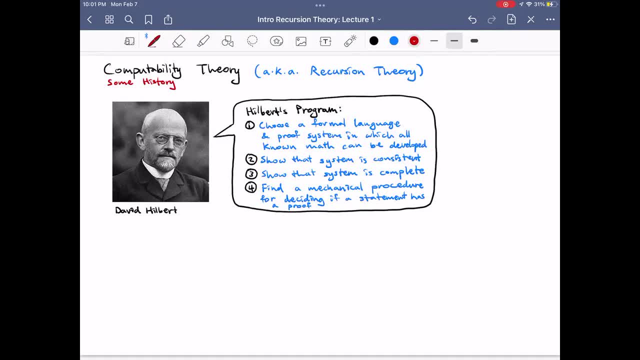 And so I want to start by mentioning Hilbert's program. So the mathematician David Hilbert had this idea that maybe you could do the following in math: You could choose some kind of formal language and proof system and then develop all known math within that formal system. 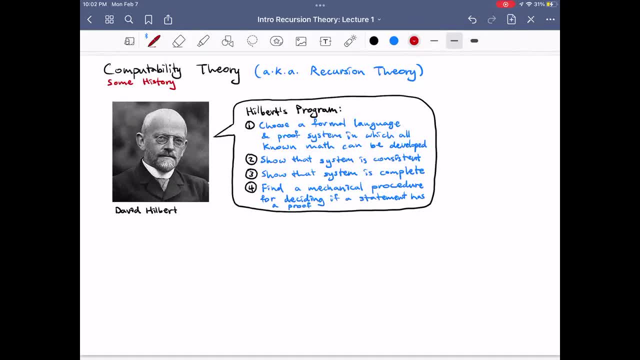 Second, maybe you could then show that the system is consistent, so you could prove that that system will never prove contradictory statements. Then maybe you could show that that system is complete. so it actually will. every statement is either provable or disprovable in that system. 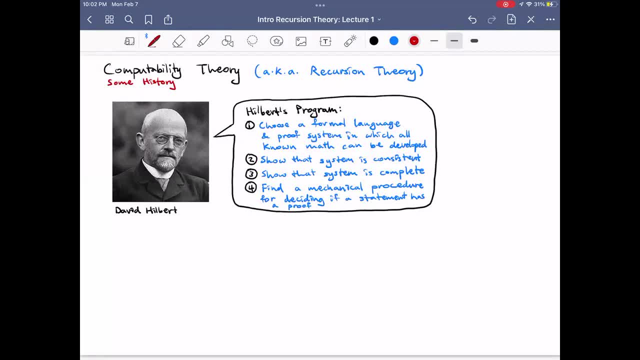 And then finally, maybe you could actually come up with a sort of mechanical procedure for deciding which statements are provable. And if you could do that you would sort of completely replace the human part of math in some way. You would have made it, you would have completely solved the problem. 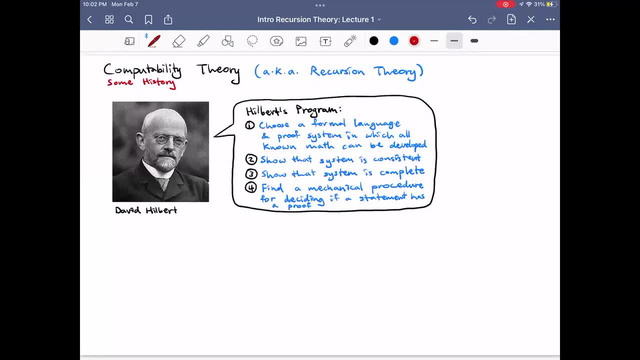 For every mathematical statement, you could state it precisely and figure out whether it was true. The first step in this program was basically accomplished with the development of CFC, set theory and first order logic. So if you've been going to the or if you go to the other courses, I think in this, in this series. 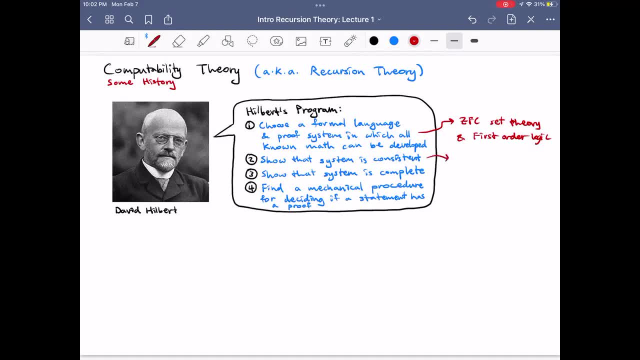 you'll see some of that. The second part, as I said, means that the system can't prove any contradictions. The third part means that it every statement is either provable or disprovable. So that's the first part, And then the third part is not the problem. 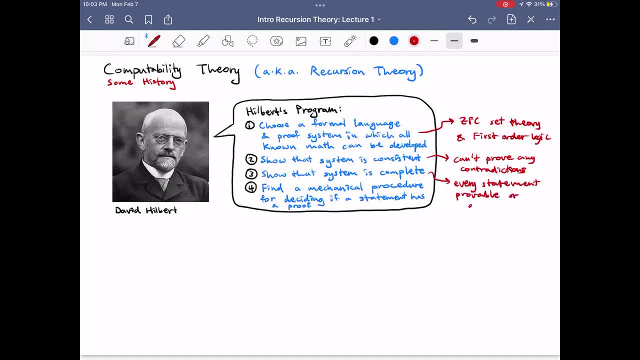 it's the��는 problem. So there's there's this whole line of the algorithm problem and it's something that's called an Einstein problem and it's begitling. And then you also have this third part, which I think um. 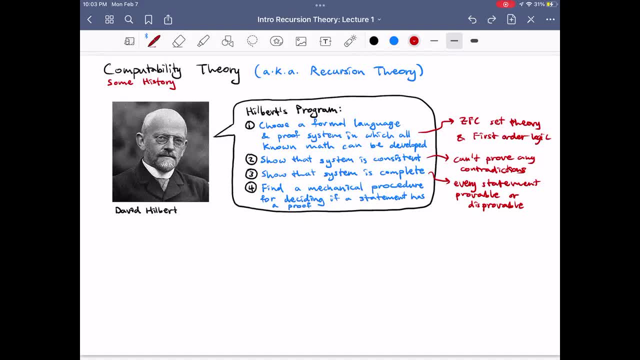 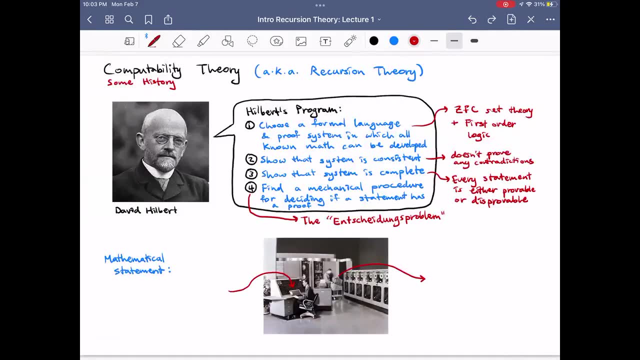 is actually, then it's called the Einstein problem. if you want to call it that way, you can call that the Einstein's problem or something like that. I'm not going to try to remember how to spell it, So that was, uh, Hilbert's program. 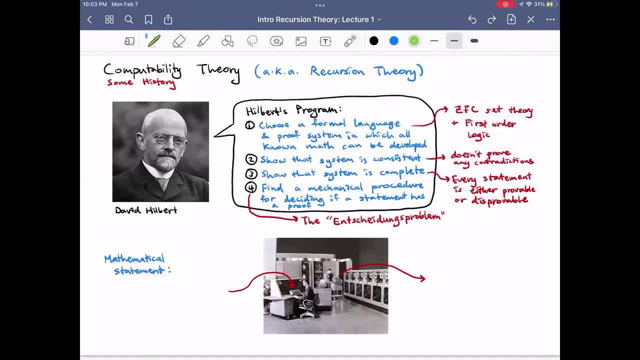 although computers didn't exist at the time- And you write down any mathematical statement, like for instance, for all n greater than or equal to three, for all a, b, c in the integers. if they're all non-zero, then a to the n plus b to the n is not equal to c to the n. 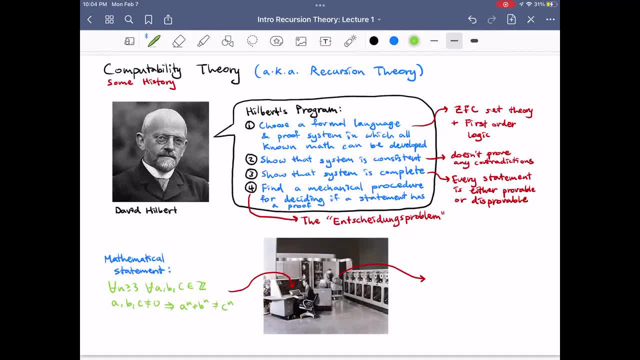 So that's the statement of Fermat's Last Theorem- And you feed it into this machine, the machine chugs along for a while and then eventually produces the result, which, in this case, is provable, And instead of waiting 300 years to find out, 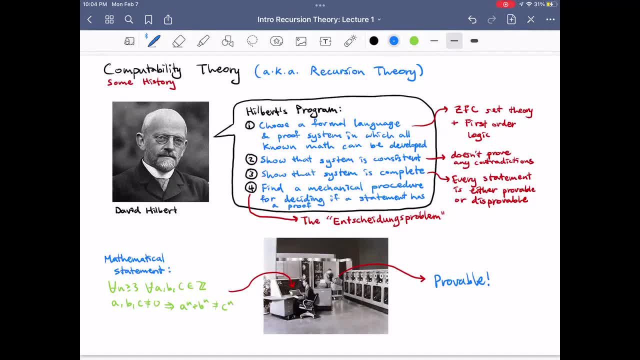 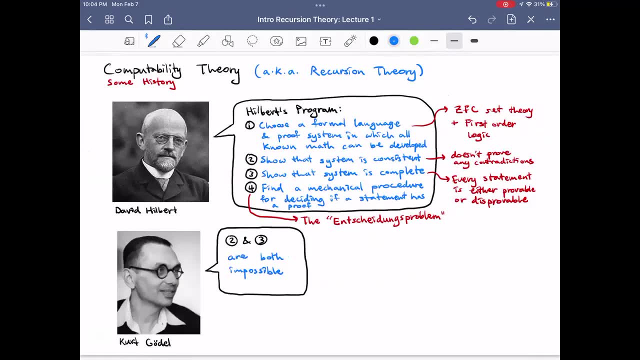 if Fermat's Last Theorem is provable, you would just immediately know. So that was Hilbert's dream. Unfortunately. first Gödel showed, that two and three in this program are impossible, And a little bit after that Alan Turing showed that number four is also impossible. 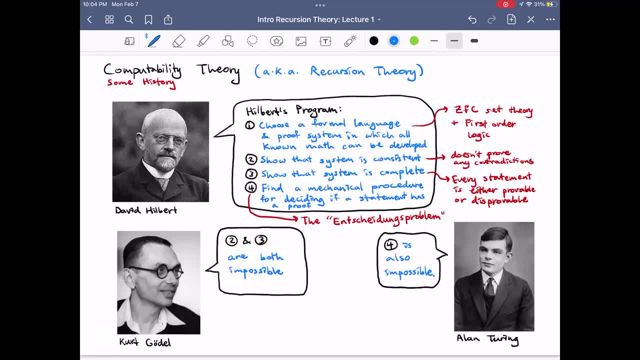 And that's really the origin of computability theory- is Turing's proof that number four is impossible. And the point of all this is to show that number four is impossible. what do you really need to do? you need to actually give a mathematically precise definition. 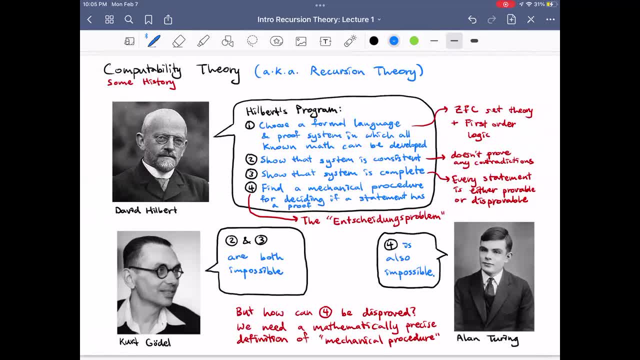 of mechanical procedure or computable or whatever, so that you can actually prove things about it. Otherwise this is just on the level of some sort of philosophical statement or something. So the beginning of computability theory was Turing's formal definition of computable. 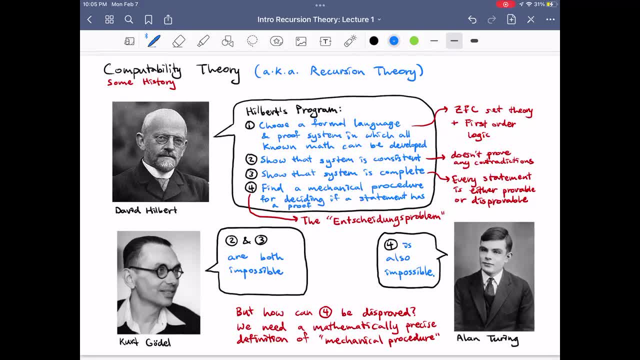 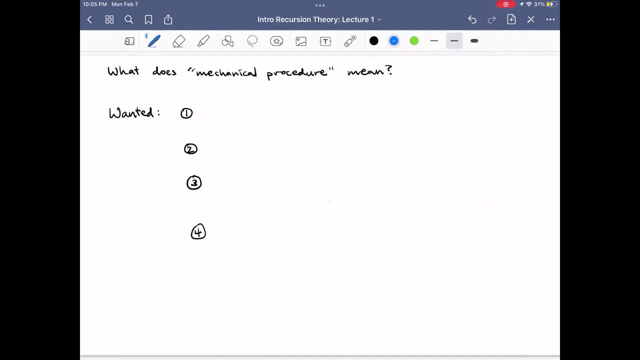 he could actually prove that this is not possible. and then subsequently people proved a lot of things about what's computable and what's not, and so on and so forth. so that's the origin of computability theory, which is also called recursion theory. um, so let's talk about what. 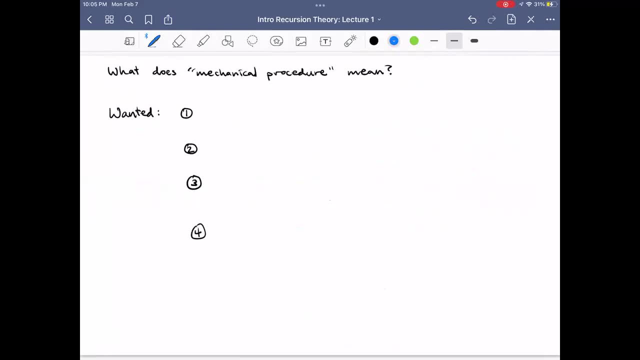 does a mechanical procedure mean? well, what do we want from a formal mathematical definition of this? uh, first, we want a mathematically precise definition that we can actually prove things about. second, we want to know that definition actually corresponds to what we intuitively mean by computable. so we want some kind of- maybe a philosophical- argument for why that definition is. 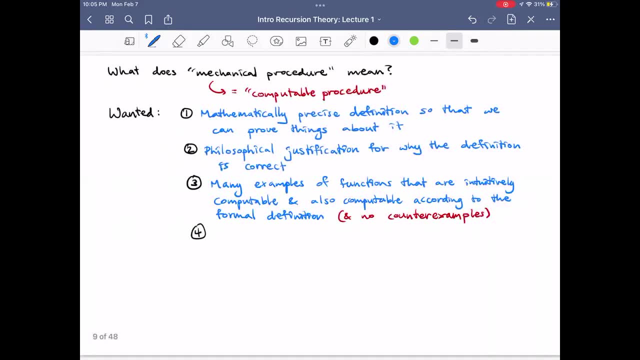 is reasonable. uh, next, um, it's maybe reassuring if you, if we can actually prove that a lot of functions which are intuitively computable are also computable according to our formal definition, and also if we try to to show that lots of such functions are formally computable. if we don't. 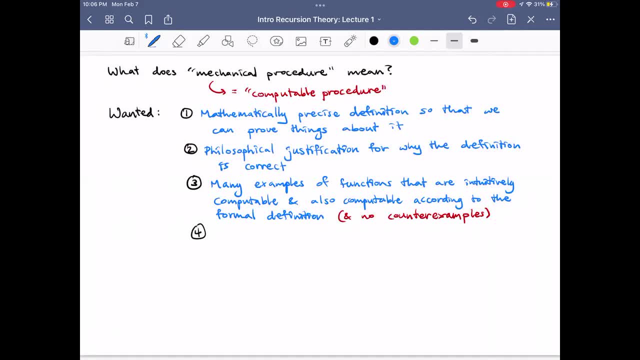 don't come up with any counter examples. that's also reassuring. So if we don't find any functions which are intuitively computable but not according to this formal definition, And then, finally, if there are multiple different approaches that all yield the same definition, 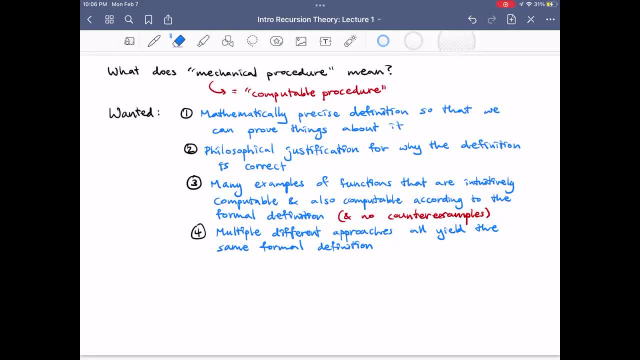 So that will reassure us that like this is kind of a very natural notion And it wasn't just some quirk of the exact definition we used. And it turns out that, at least most people's opinion, all of these things have been achieved. So let me just mention number four. Around the same time. 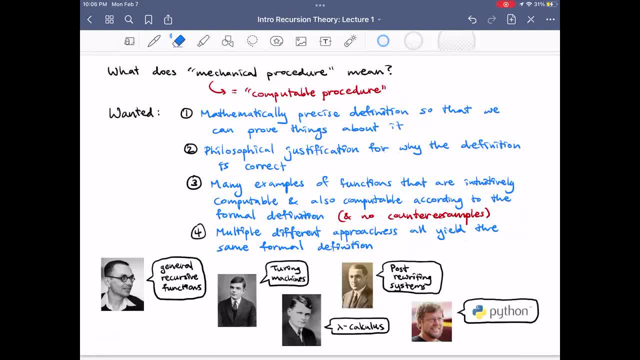 a lot of different people gave definitions, formal definitions of computability. So Goodall defined something called the general recursive functions, Turing defined something which are now called Turing machines. He didn't call them that. There was lambda calculus, post-rewriting systems and so on. And now in the modern day, of course there's a million. 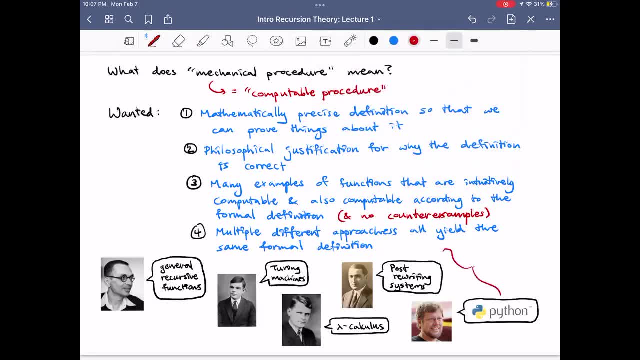 programming languages, And it turns out that all these things are equivalent. And, furthermore, what was Turing's biggest contribution? So it actually turns out some of these things were defined before Turing defined Turing machines. But his great contribution, I would say, in this aspect at least, is- at least one of his contributions- was giving the most. 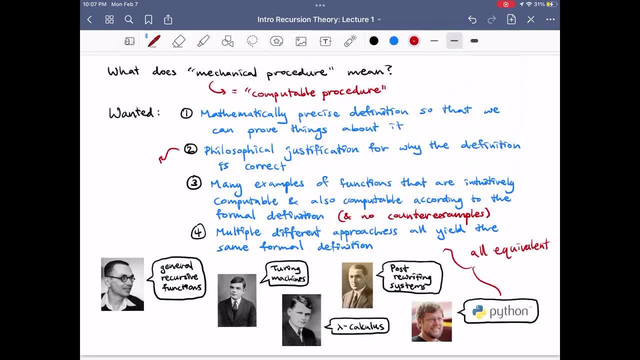 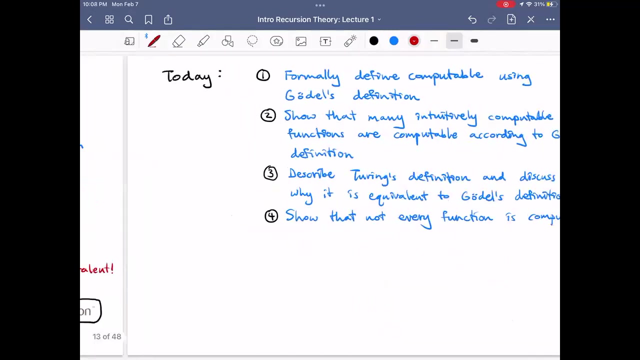 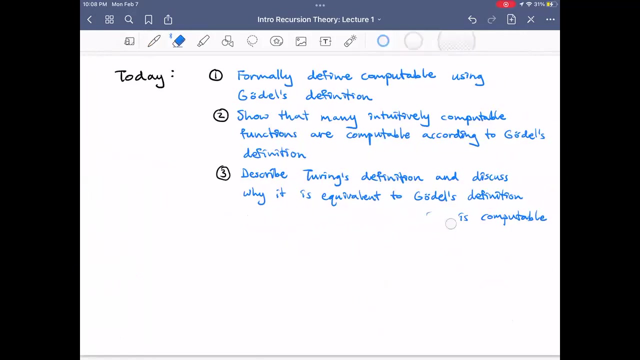 compelling philosophical justification That his definition was correct. Okay, So that's kind of a brief overview. So what am I going to try to talk about today? Actually, I'm going to skip this, This last part, for now. So I'm going to try to formally define computable using, actually, 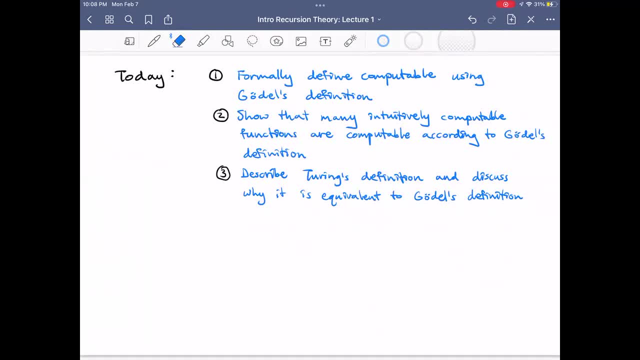 Goodall's definition, which I said was this general recursive function definition. We're going to do that because that definition is easier to work with, sometimes easier to prove things about, requires less cumbersome notation and so on. Then I'm going to give you some examples to 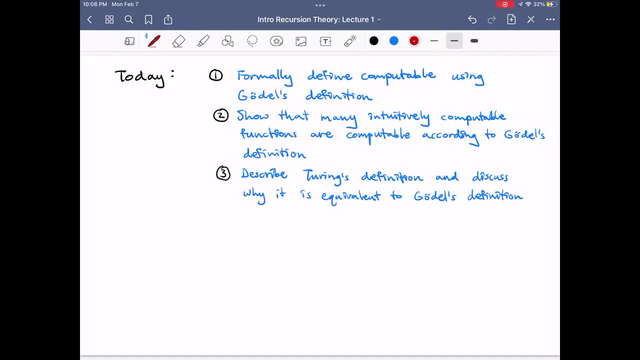 show that at least some intuitively computable functions are also computable according to Goodall's definition, In other words, they are general recursive functions. And then, finally, I want to at least briefly describe Turing's definition and why he argued that it's a sort of correct definition of computable. 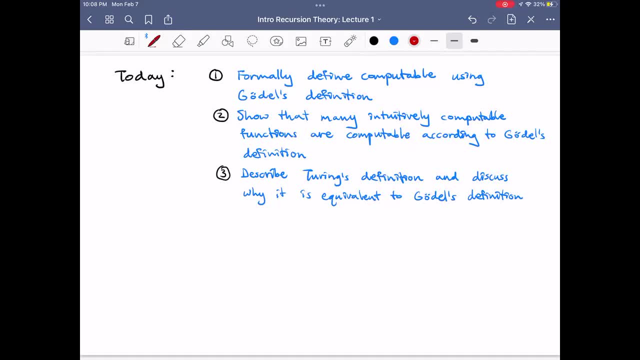 and briefly mention how you can show it's equivalent to Goodall's definition. So that's basically the plan for today, And then maybe in the next session I'll do this last item. So let me remove it for now. And as a final comment: in the modern day I think many people have experience with programming. 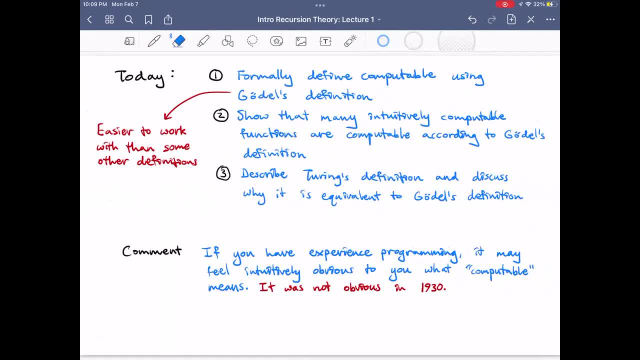 languages. So many people have done a little bit of coding And if you've done that, sometimes it feels like why do we need to spend much time setting up a definition of formal computability and justifying that it's invalid and so on? Because I don't know if you've programmed a bit. 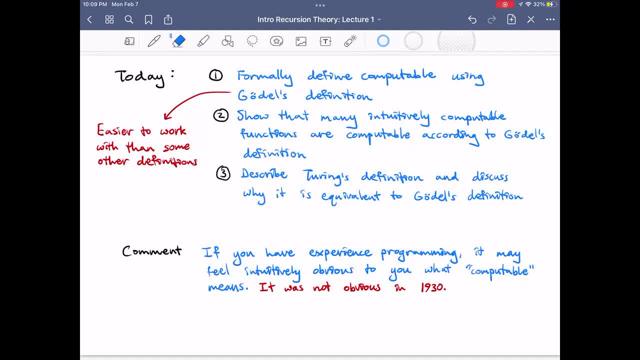 you just feel like you know what it means for something to be computable, You know what it means to be able to write a Java program that does something, or a Python program or whatever. But the time that Turing was working, this was not really obvious at all. So in 1930,, 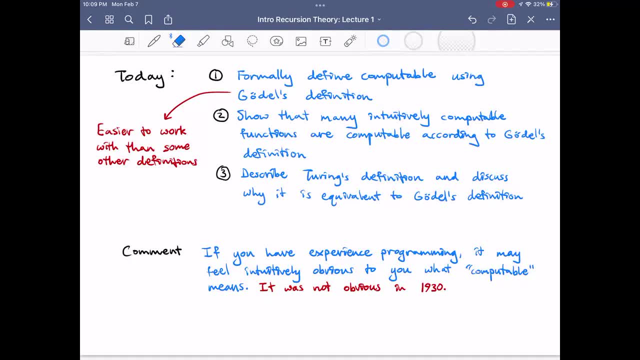 computers did not exist. No programming language had ever been invented- really Well, maybe, but not really, And so it really wasn't obvious at all to people what computable meant formally. So David Hubbard had never seen a programming language or a computer or code or anything. 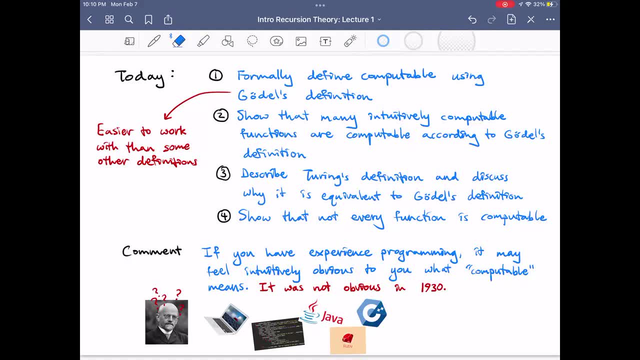 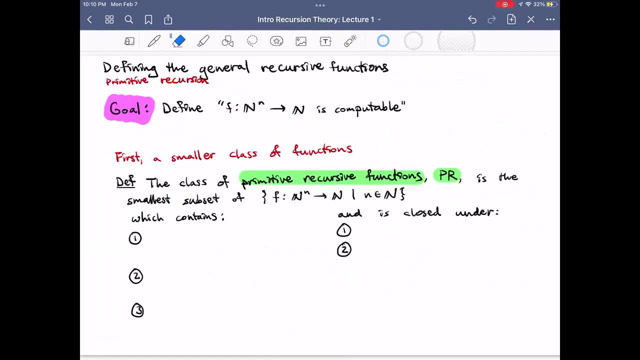 Okay, So that's the setup. Now we're going to switch to some more sort of technical details. So this is kind of the overview And, by the way, feel free to let me know if you have questions or if I'm going too fast or too slowly or anything. Okay, So we're going to start as I said. 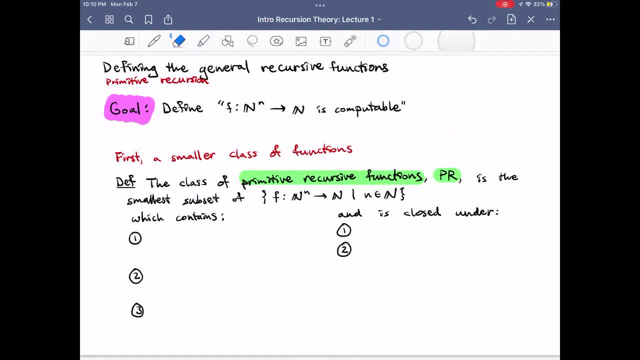 with defining Gödel's definition of computable, And that's actually going to take up most of the time. So, in particular, what we're actually going to define is what it means for a function which takes natural numbers. So it takes natural numbers as inputs and gives you a natural number as output. what it means for 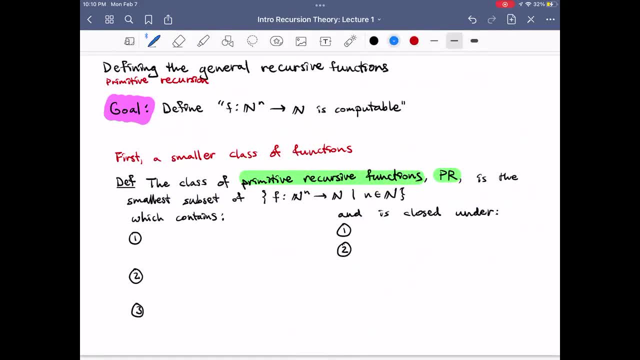 that to be computable. And in case you think this is sort of too narrow, like: why should we only allow natural numbers as input or output? it's easy to switch to other domains, For instance infinite binary or, sorry, the arbitrarily long. 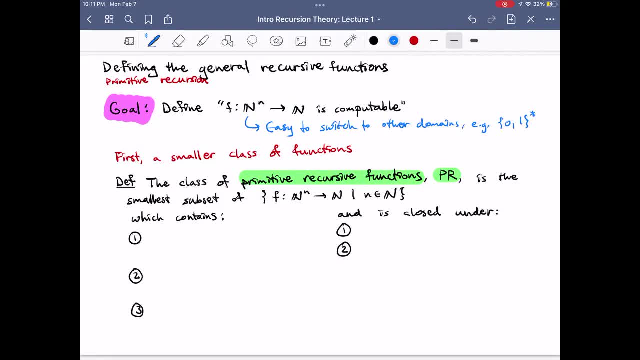 binary sequences arbitrarily long, finite binary sequences, which you sometimes see denoted like this. So once you set up this definition, it's not that hard to change what the domain is. But just for the sake of concreteness, let's stick with this particular setting. So we're going to 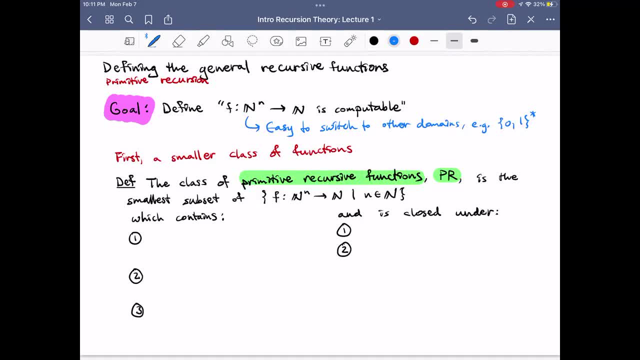 define computability of functions on the natural numbers to the natural numbers And in Gödel's definition it's actually convenient to first define a somewhat smaller class of functions which turns out to be smaller than the classic Computable functions. So everything in the class we're about to find is computable. 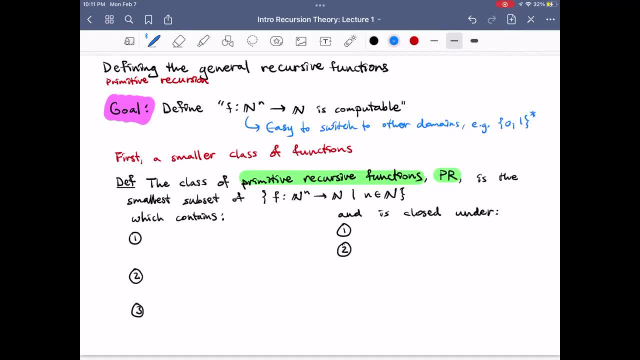 but it doesn't cover all the computable functions, And this class is sometimes called the primitive recursive functions- I'm going to abbreviate it PR- And it's defined as the smallest class of functions from natural numbers to natural numbers, which contains three functions and 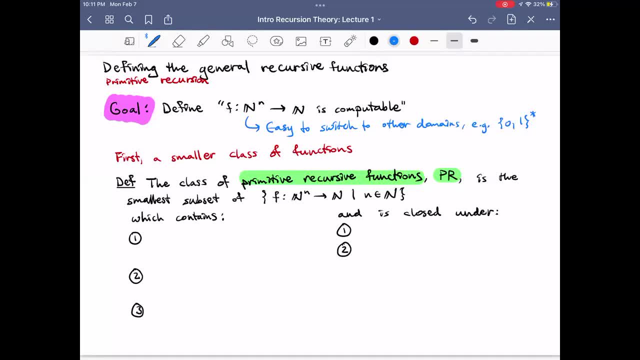 is closed under two operations. So the three types of functions it contains is constant functions, The successor function and projections. And now I'm going to say what each of those are. So the constant functions, these are functions that maybe I shouldn't say it like this. Here's one example of a constant function. 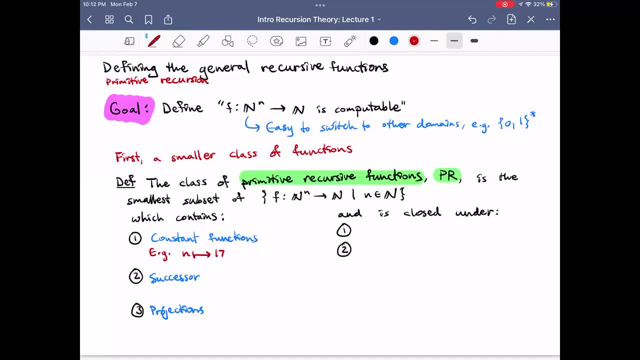 It takes an input n and it just always gives you the number 17.. So this is the constant function with value 17.. I'm going to sometimes denote that c17, c18.. Next, the successor function. This is just the function that takes a number. 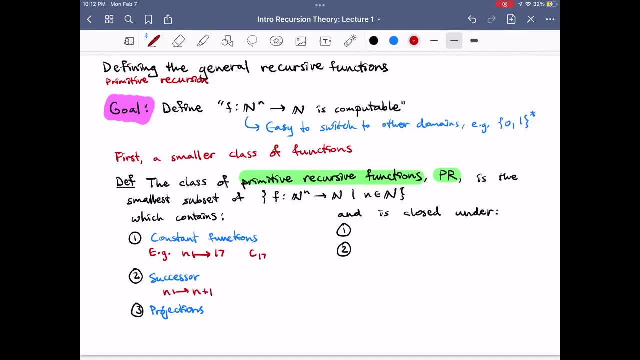 and gives you that number plus one. And finally, projections. These are functions that take multiple inputs, So they might take, like, four inputs: n1,, n2,, n3, and n4. And they just always give you the same one of those inputs. So maybe this projection function always gives you n3. 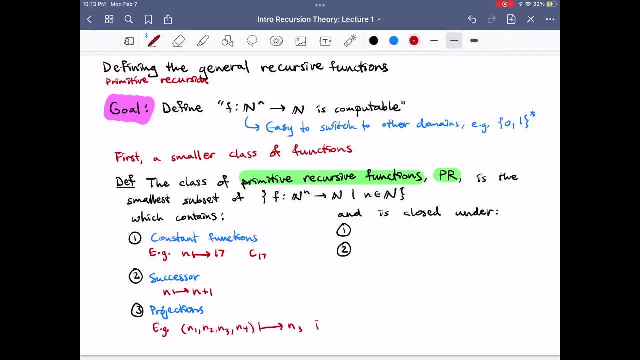 So it takes four numbers and gives you the third of those numbers. And I'm going to denote this. p43 to denote: it takes four inputs and gives you the third of them. So these are all like very simple functions, obviously computable. So they're all counted. 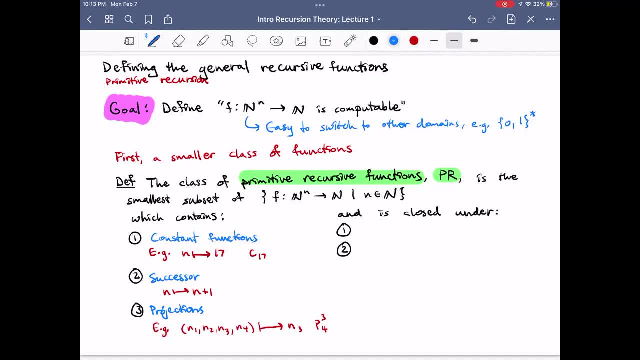 as primitive recursive, And then the set of primitive recursive functions is closed under these two operations. First something sometimes called composition or also sometimes called substitution, And then another operation called primitive recursion. And in case you're not sure what those terms mean, I'm going to define them in the next couple. 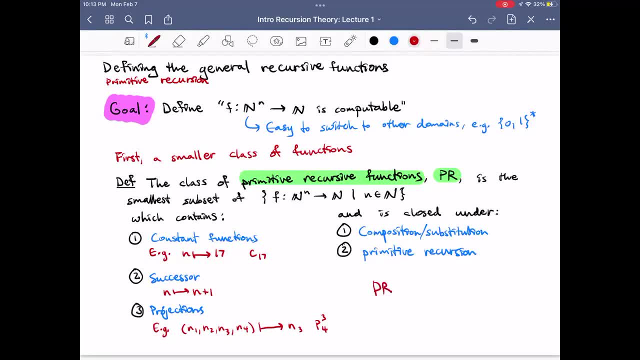 slides. And then, more formally, you can define the set of primitive recursive functions as the intersection of all sets of functions which contain these ones on the left and are closed under the operations on the right. So if you want to prove that, um, some class of functions contains all the primitive recursive, 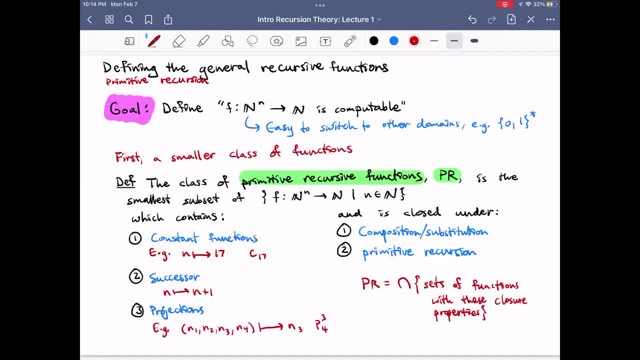 functions. one thing you can do is show that it contains these functions on the left and it's closed under the operations on the right. Buchanan, gentlemen, be referenced by the geological factors as the Einstein theorem issociationally unsure and strangely, that I relationships. 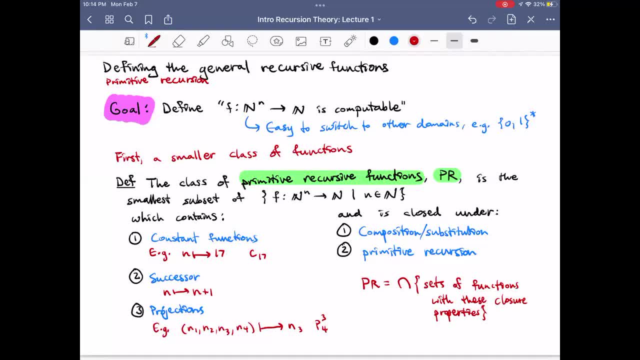 å. So if you want to prove that, um, some class of functions contains all the primitive recursive functions, one thing you can do is show that it contains these functions on the left and it's closed of the computable functions. So that's why all primitive recursive functions 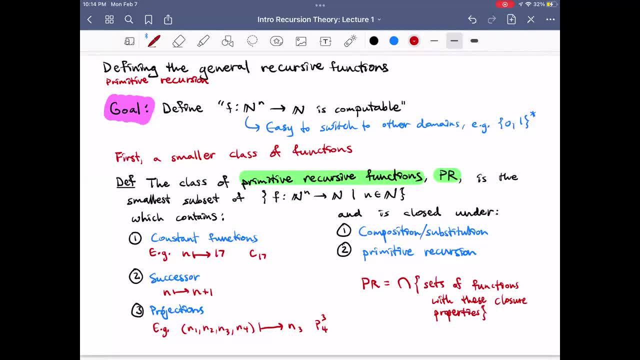 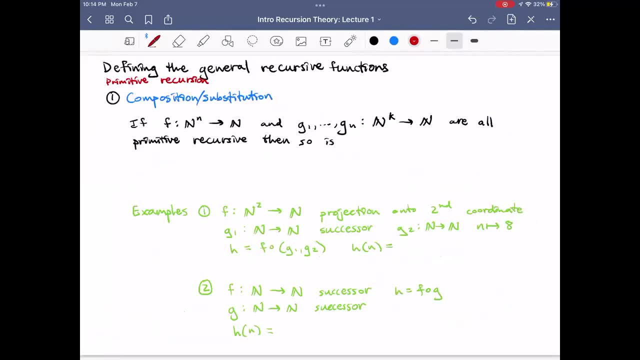 are computable. So now I'm going to describe composition and primitive recursion. So composition, this is the principle. If you have a function f from which takes little n inputs, and then functions g1 through gn which each take k inputs, 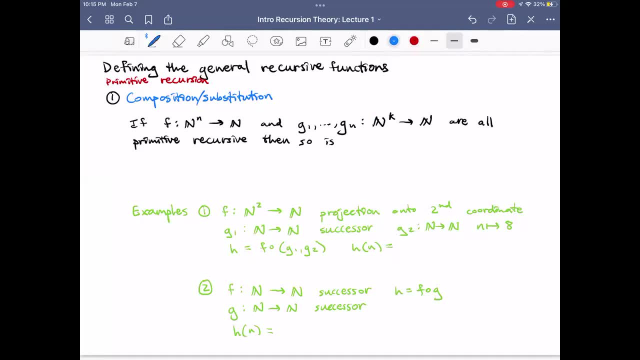 if they're all primitive recursive, then so is the following function, The function that takes k inputs and given k natural numbers, what output does it give you? It gives you f, with f's first argument is g1 of n1, through nk and so on. 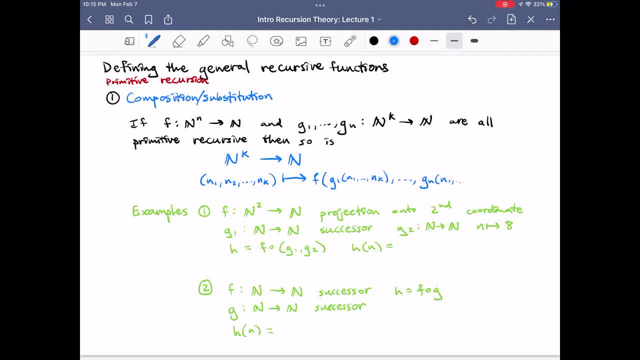 So first you apply all the functions, little g, to the input, and then you apply after that, And sometimes I'm going to denote this as f composed with g1 through gn, So I'll use that notation. So let me just do a couple examples to clarify the notation. 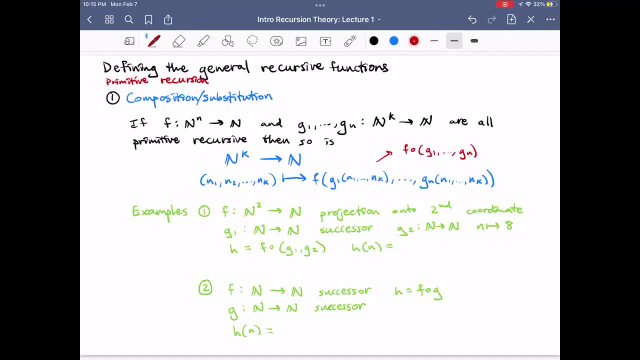 So suppose you have, I don't know, I don't know, I don't know You have. f is the projection onto the second coordinate. So remember we had all projections and g1 is the successor function and g2 is the constant function with a value eight. 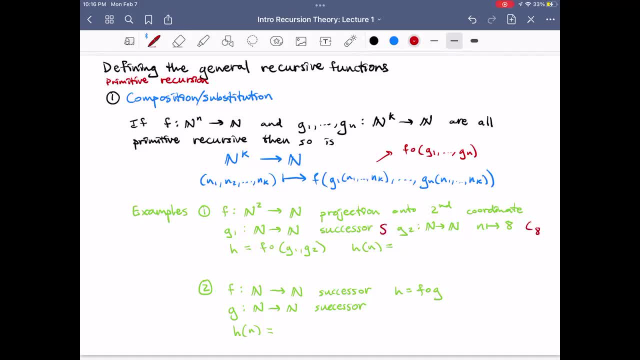 And I should say I'm going to denote successor sometimes as s. So let's see what is h of f composed of g1, g2? Well, h of little n is going to be f of g1 of n comma, g2 of n. 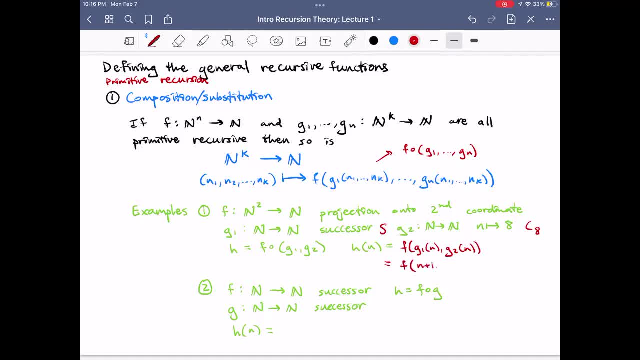 g, one of n, that's the successor, so that's going to be n plus one, and g2 of n, That's always equal to eight. So the constant function, and now f- is projection to the second coordinate, which means it just gives us the second of its inputs. 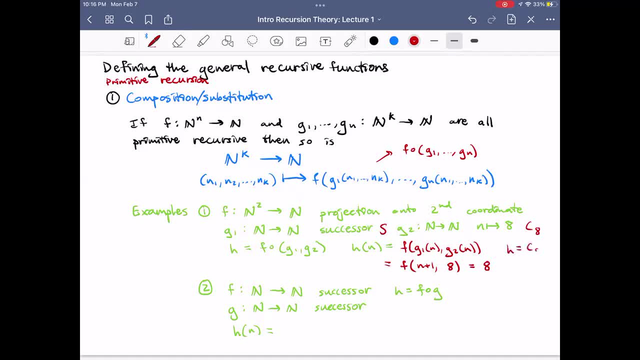 So it's equal to eight. So in fact here h is also equal to C a. So we didn't get anything new by applying composition here. but that's what composition does. Now let's see a case. So we do get something we didn't have before. 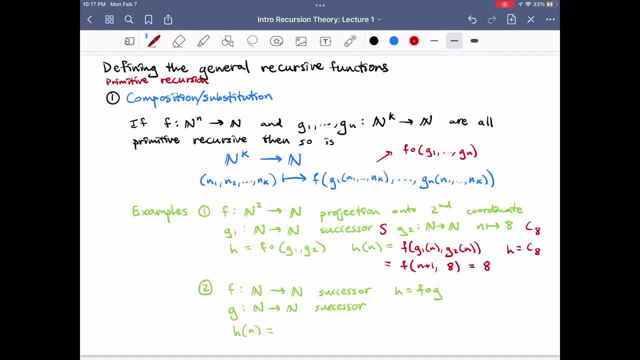 Let's say f and g are both the successor function. So in this case, like little n would be one and little k would also be one. Here, what is h of n? Well, it gives us f of g, of n, which is f of n plus one. 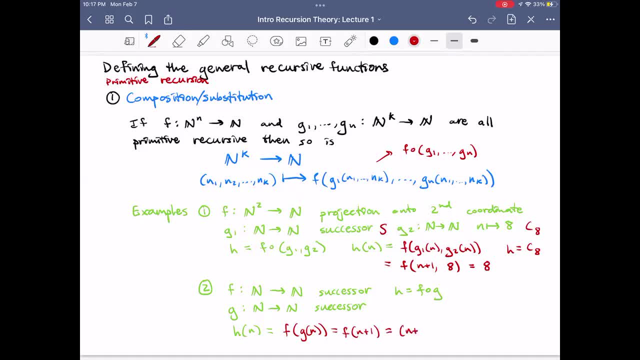 And f gives us the successor of that, which is n plus one plus one, In other words n plus two, And by induction you could actually show for every n. the function m maps to m plus n is primitive recursive, So you just compose the successor function. 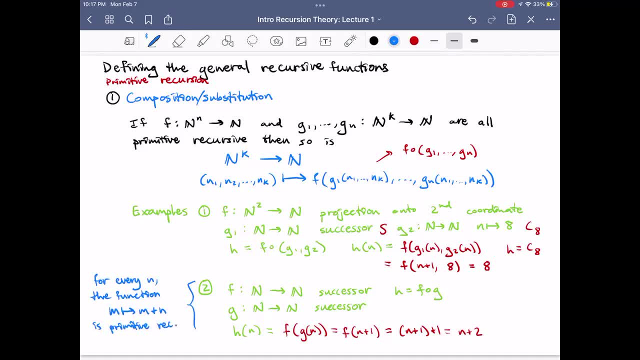 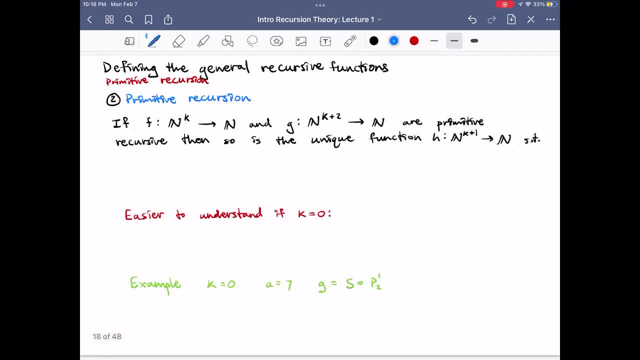 with itself n times, and you'll get this Because of the Sequdel complication. make sure that's in subdivision. So that's how composition and substitution work. Let me now describe primitive recursion. So this one kind of looks funny at first, I think. 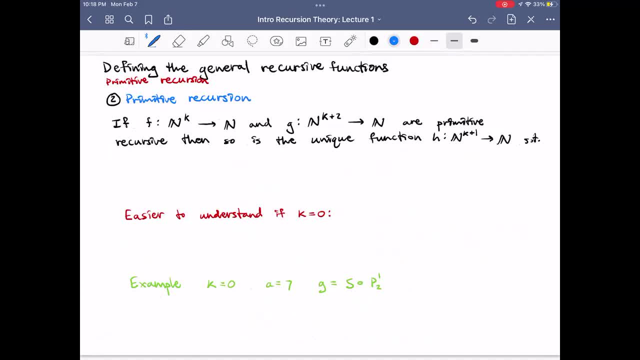 but the idea of it is not so complicated once you get past annotation. So in primitive recursion you have two functions, a little f and little g, and the first takes k inputs and the second takes k plus two inputs And you get a function that takes k plus one. close to me. 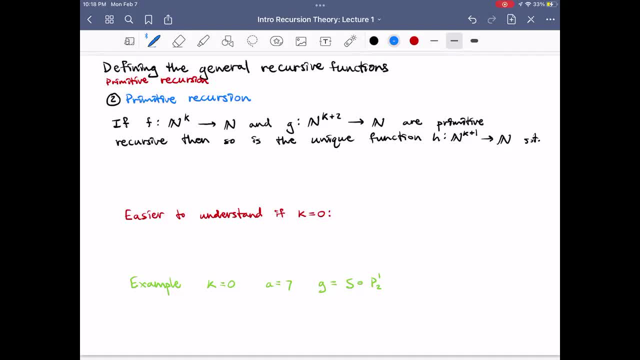 Just the last step. So you get a function that comes out, and then I get the rehabilitation of the 79. k plus one inputs, and it has the property that when the first input is zero, it's just doing exactly what f does. 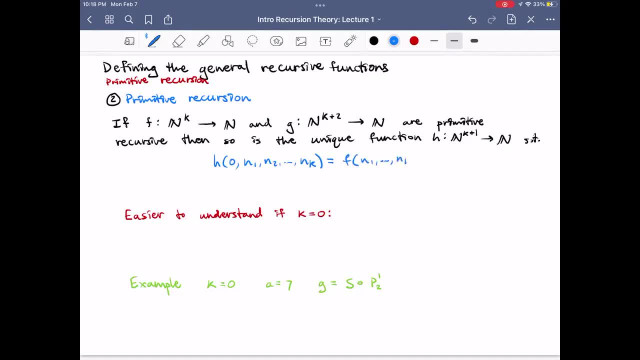 with the rest of the inputs And for every other input. if the input is n plus one, then g tells it what to do, And in telling it what to do it uses the previous value of h. So h is the unique function. 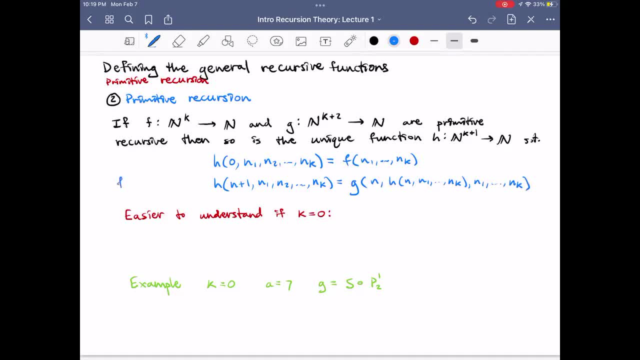 that satisfies these two properties. The second property is for any n in the natural numbers. So you can show by induction that h there is a unique such h, and the primitive recursion says: if little f and little g are primitive recursive, then so is this function little h. 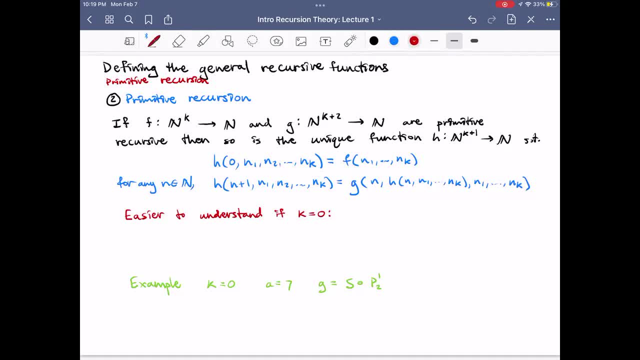 And you should think this is some form of recursion, because in defining one value of little h we're using some other value of little h. So you can kind of think we're recursing or we're making some recursive call to little h. We're making some recursive call to little h. 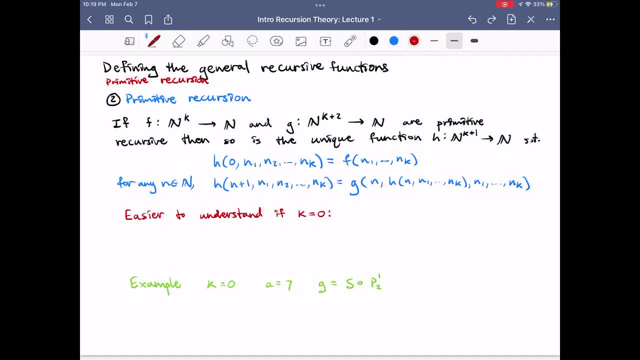 with n instead of n plus one. Okay- and this is maybe easier to understand- if you set k equal to zero and just ignore all these extra inputs, Although sometimes we will use larger values of k. So if k equals zero, f is a function that takes no inputs. 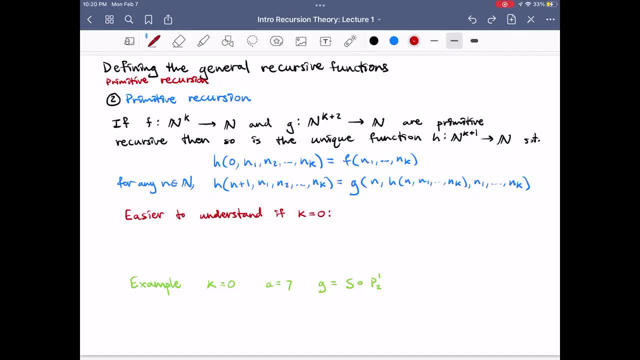 So it's actually just has to be a constant. So in that case it's saying something like h of zero, is this constant? a, Let's say, and h of n plus one is equal to g of n, comma h of n. So it's saying like, at zero, you just get this constant. 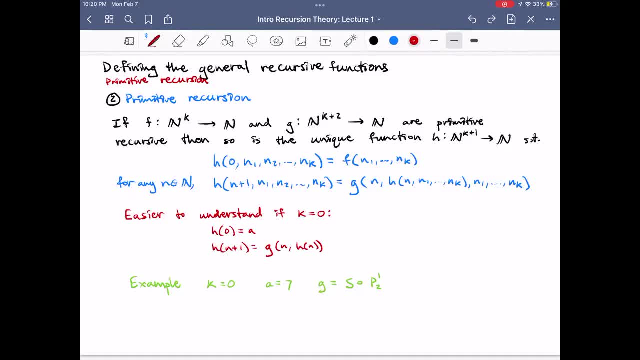 and the next value, g, tells you how to get that value from the previous value, and so on. So that's the idea of primitive recursion. And now let's do an example again with k equals zero, So with like no extra inputs, Although, again, often you do want to have these extra inputs. 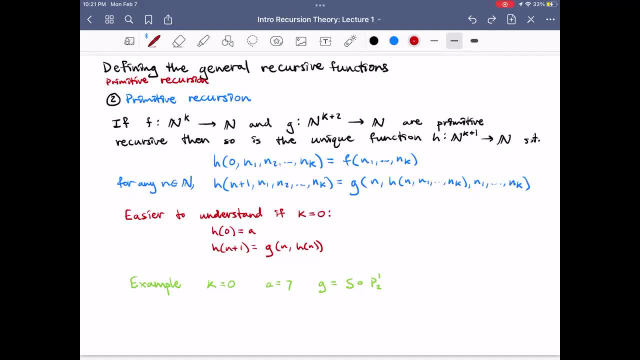 So in the example let's say the starting value is seven and the function g is the successor function composed with projection onto the first coordinate. So first let's try to figure out what g is doing. So remember g should take two inputs, n and m. 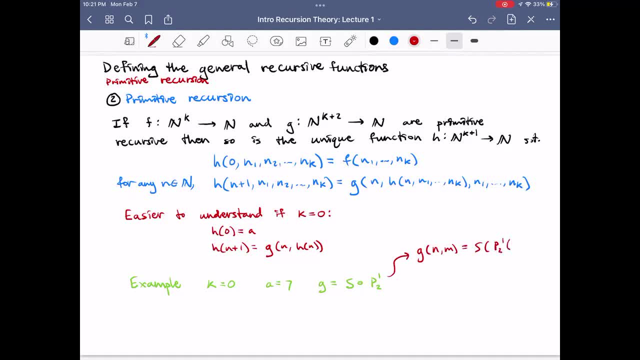 and it's going to give us the successor function of p21, of nm And the success. well, p projection onto the first coordinate is just going to give us n. So the successor to this is going to just be: this is just going to give us n plus one. 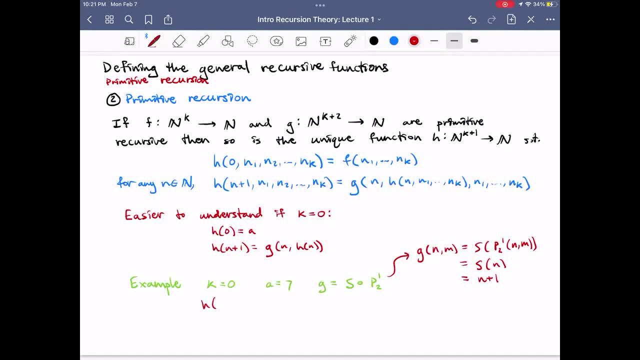 So, in other words, this is going to give us n plus one. So in other words- sorry, I think that I made a typo here And what I meant to say was projection onto the second coordinate. So if we change that, I think this will become a more interesting example. 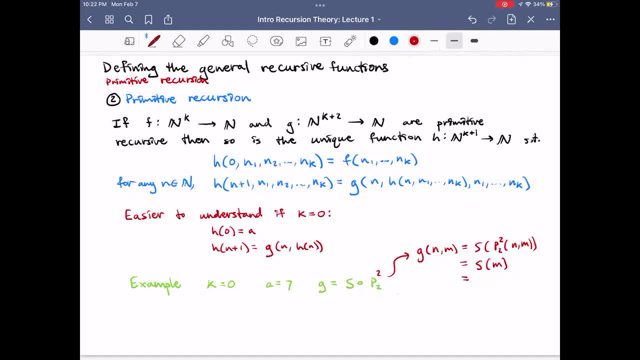 So, projection, the second coordinate will give us m, and this will be m plus one, And what we'll do is we'll take the successor. It will become a second coordinate, a second coordinate. We'll call it h of two. So this is going to be h of a. 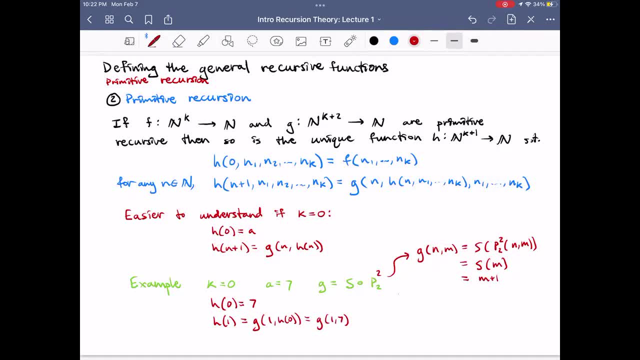 This is going to be a second coordinate, which is a second coordinate, And the second coordinate is g of one, which is g of two comma h of zero, which is g of one comma zero. And what does g do? It takes the successor of the second coordinate. 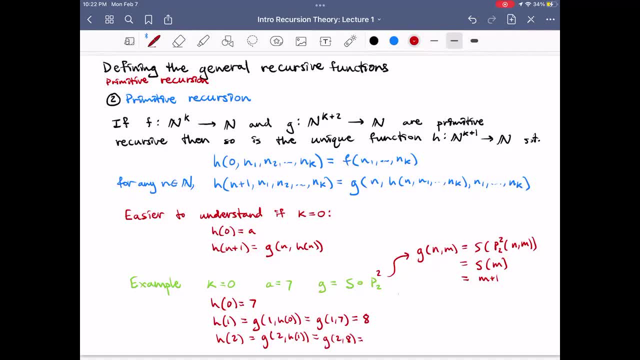 So this is going to be h of two. g will take the successor of the second coordinate, so it will be 9.. And you can continue like this and see in general, h of n is actually going to be n plus 7.. Okay, so that's how primitive recursion works. We're going to do more examples, so hopefully, 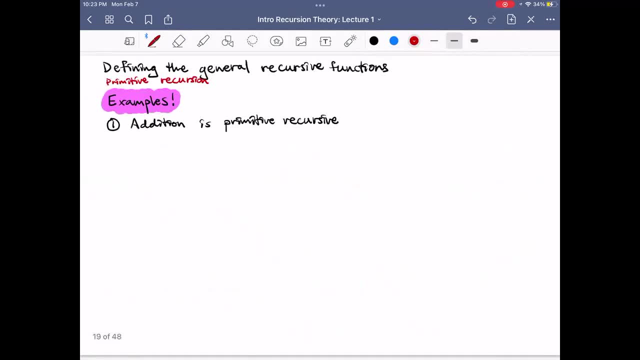 it will become clearer gradually how it works. So yeah, so let's see some examples. So now we're basically just going to verify that a bunch of different functions are indeed primitive recursive. So first let's check that addition is primitive recursive. So the 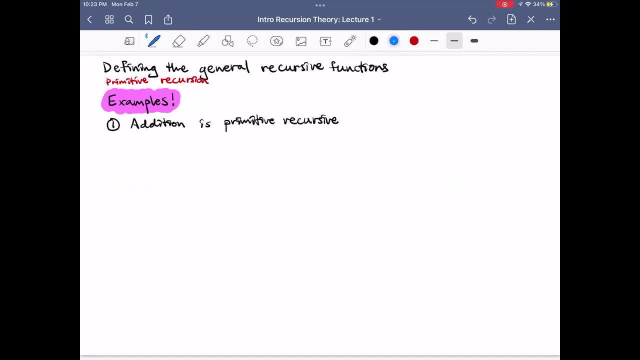 basic idea is that we want to define some function like h of n m equals n plus m. So how can we define this by primitive recursion? Well, first we're going to say h of n m equals presto, and 0 is equal to just. should be just equal to n And h of n comma. 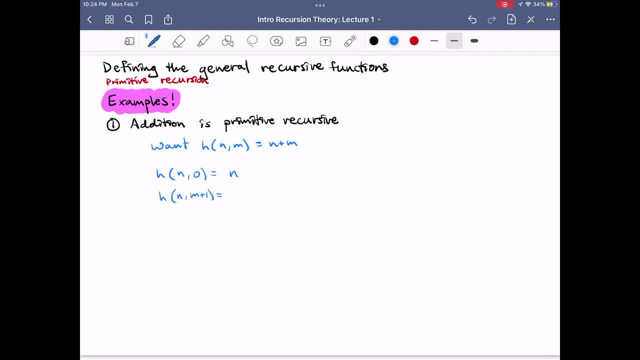 m plus 1 should be equal to…. Well, n plus m. Okay, Okay, great, Okay, Okay, Okay Okay, m plus one. but if you put the parentheses in a different place, you see that we could really replace h of n plus m- i'm sorry, m plus m with h of m m, so in other words, this is sort of a. 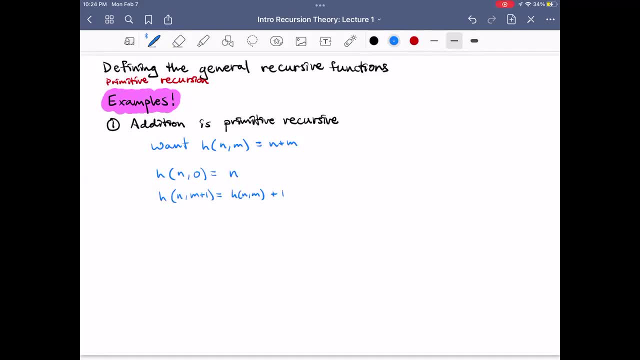 recursive definition of addition. the n plus zero is n and n plus m plus one is n plus m plus one. but now we need to fit this into the framework of primitive recursion. so we're going to apply primitive recursion to get this with k equal to one and our starting function f. well, it should be. 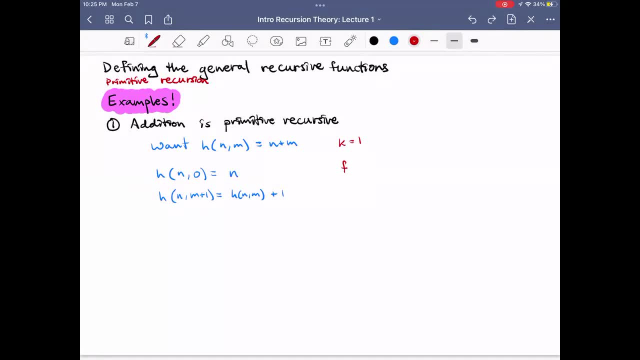 i guess ignoring this, this input. so maybe to fit into the way i literally defined things earlier, i want to switch the order of these two. so i want to say like zero n and something like this. i just had the order backwards from before. okay, so little f should take one input, n, and it should just give us n back. 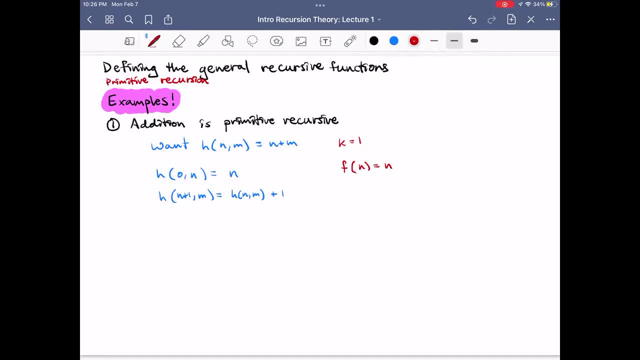 and you might be worried. we don't actually have that function. that's the identity function. but we do have it because it's the projection of one input onto the first coordinate. so p one, one of n just always gives us n. in other words, it's the identity function. 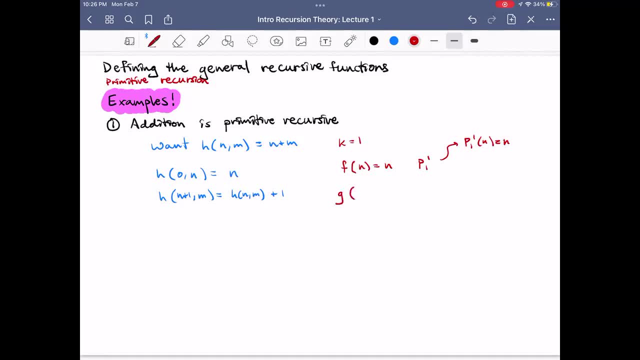 and then, what should our function, little g be? so little g is supposed to take a number n and a value a, which you should think corresponds to h of n, m, and then it takes, uh, this other argument, in this case m, and what should it give us? well, we want it to give us just a plus one. 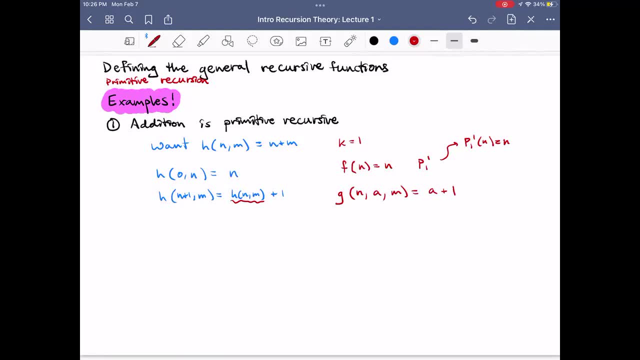 okay, so then you can check. uh, if we actually define things this way, we'll go to function a h such that h of uh zero n is equal to f of n, which is equal to n, and h of n plus one comma m is equal to g of n, comma h of n m, common m, which is h of nm plus one. and, by the way, why is it, uh, why can we do this? 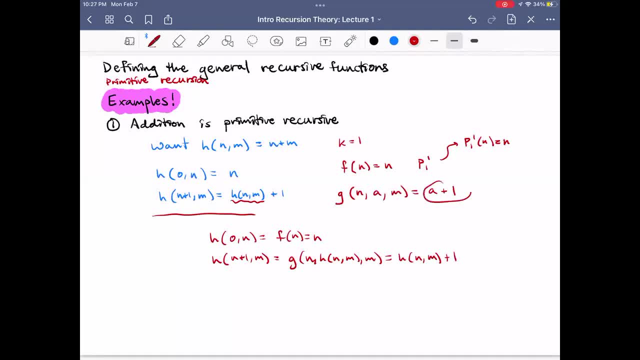 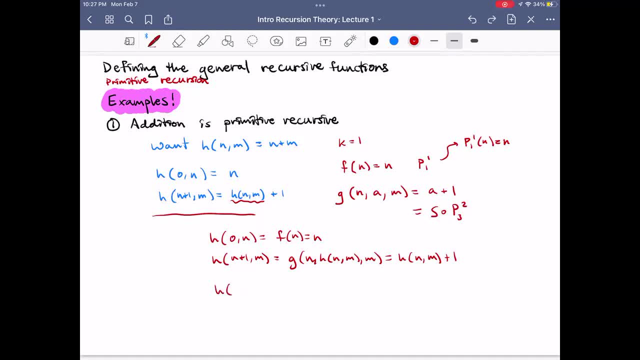 you'd see that, like H of one, N is going to be H of zero, N plus one, which is just N plus one. H of two N is going to be H of one, N plus one, which is N plus one, another plus one, so that's N plus two. 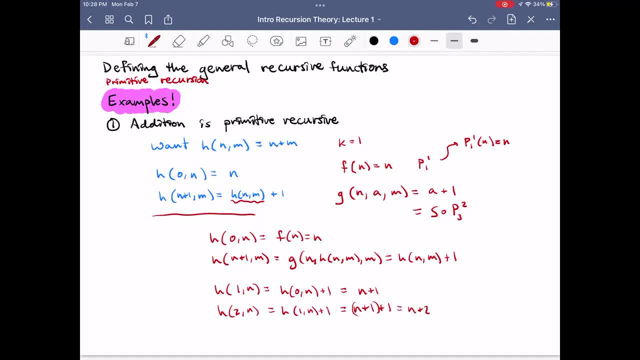 So you can then verify this really as addition. So that's how you can use primitive recursion to define addition, And since we were applying primitive recursion to functions we already know are primitive recursive, that tells us that addition is primitive recursive. Okay, So let me know if you have questions about this. 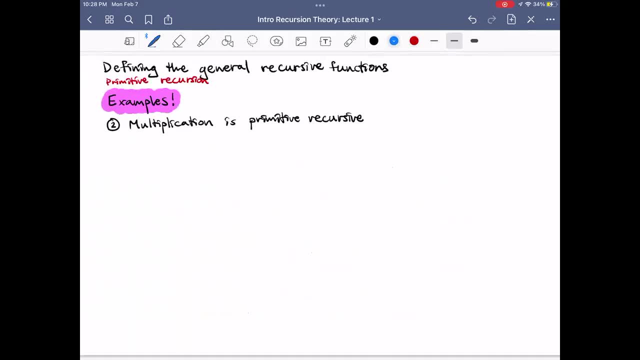 Now let's do some more examples. I'm going to go slightly faster on these. Hopefully you've started to get the idea of how primitive recursion works. So let's show that multiplication is primitive recursive. Well, the idea is: let's say we want to define H of N, M, 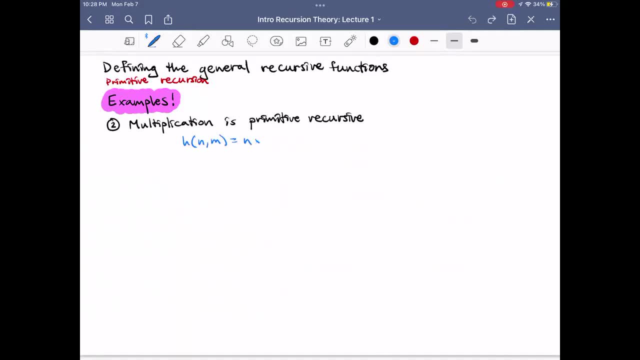 is equal to N times M. How can we do this? Well, first let's define H of zero M, So this is zero times M. This should just be equal to zero. And now let's define N plus one times M. This should be equal to what we want it to be equal to. 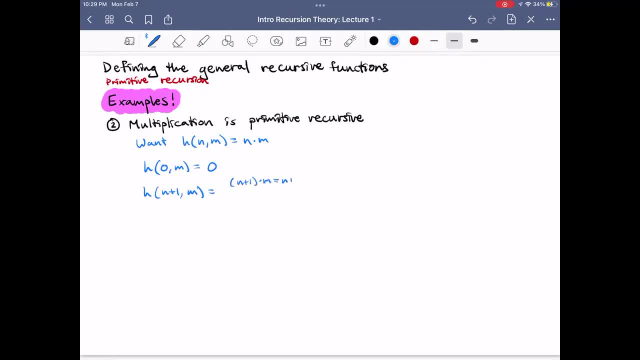 is N plus one times M, which is N M plus M. So what we should do is this: N M is what H of N M is supposed to be, So you can just write H of N? M plus M, Okay, and that's basically the entire proof. 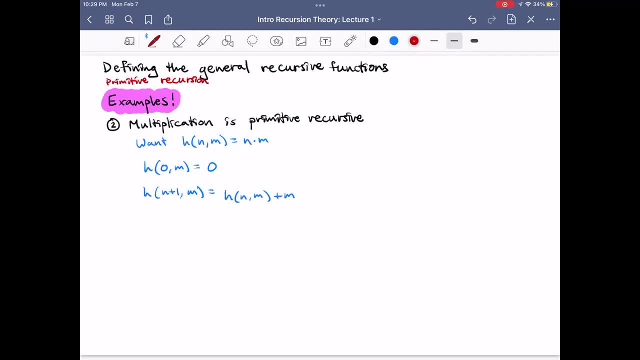 that multiplication is primitive recursive. If you want to be more formal again, what you can say is: again, we're doing primitive recursion with K equals one. little f is the constantly zero function And little g takes N, A and M and it just gives you A plus M. 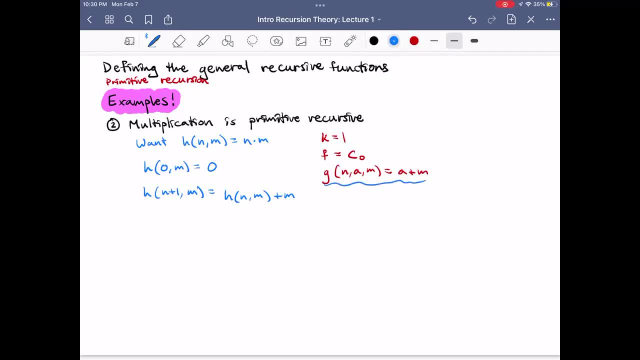 And how do we know that this function is primitive, recursive? Well, that's what we just saw. Well, more or less what we just saw. So g is equal to the function that adds two numbers together, composed with projection onto the second coordinate. 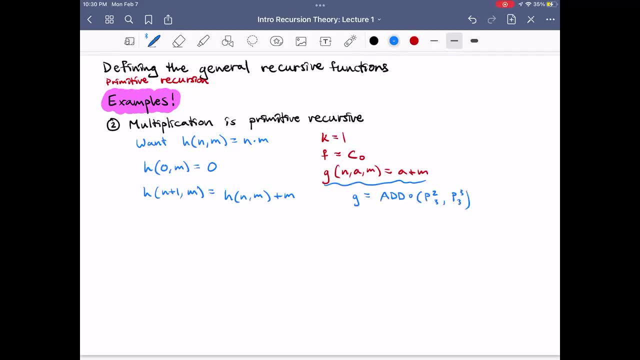 And projection onto the third coordinate. So we basically want to add together two numbers, but we have to ignore the first number we're given. So that's why multiplication is primitive recursive. Let's do maybe one more example like this. So exponentiation is primitive recursive. 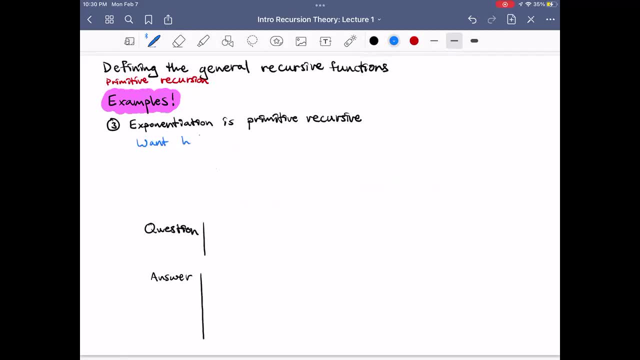 So again, we want to define H of N M to be N to the M. so we can do this by setting H of zero M. This should be well. now there's kind of a problem. This should be zero to the M. 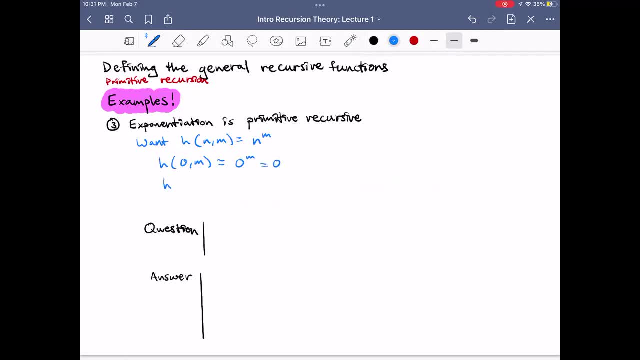 So it should be zero. But then if we try to define H of N plus one M, we would want this to be N plus one to the M, And it's maybe not so easy to define that in terms of like N to the M. 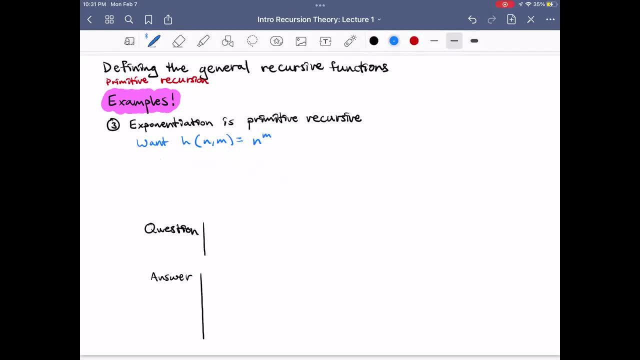 So instead, we're going to take a different approach and we're going to define it in terms of recursion. on this, the other on M instead of N. So in order, it's H of N zero. this is should be N to the zero, which is just one. 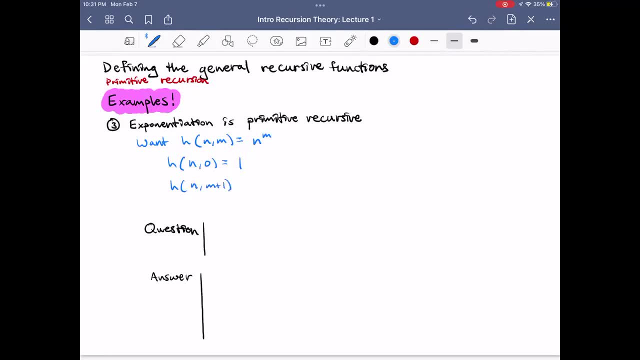 Oops, And H of N M plus one. This should be N to the M plus one, which is N M times N. So in other words, this should be H of N M times M Oops times N. So we have sort of given a definition. 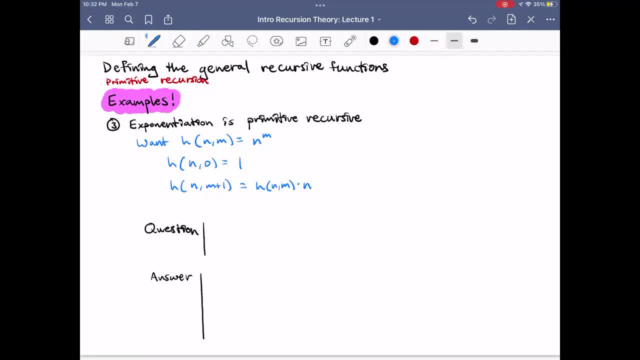 in terms of primitive recursion. except that in primitive recursion we were supposed to be doing recursion on the first input rather than the second. So we should really define: is H of N- M equals M to the N, H of zero- M equals one. and H of N plus one- M plus one. 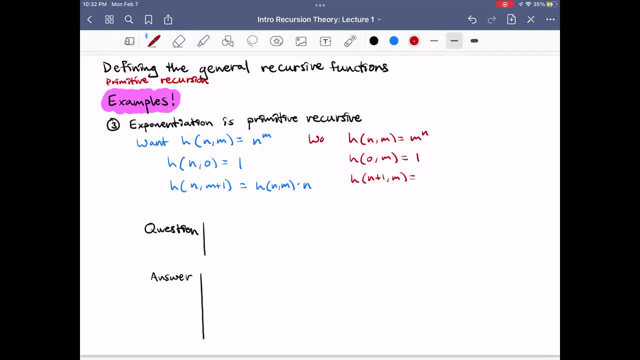 And then we have H of N- M equals H of N M times M. And then we have H of N M times M, which looks a little funny because I don't know the order of N in them are reversed from the way you would normally want to write it. 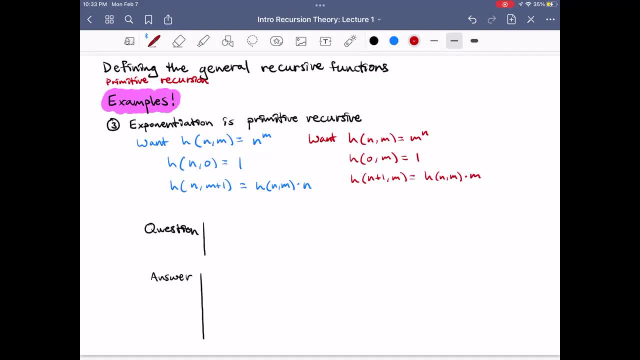 It's just a quirk of the exact way we start permanent recursion, But the question is: maybe So here, H of N, M is actually the final approach to the final method of recursion, So it should be So. this is is actually equal to m to the n instead of n to the m. 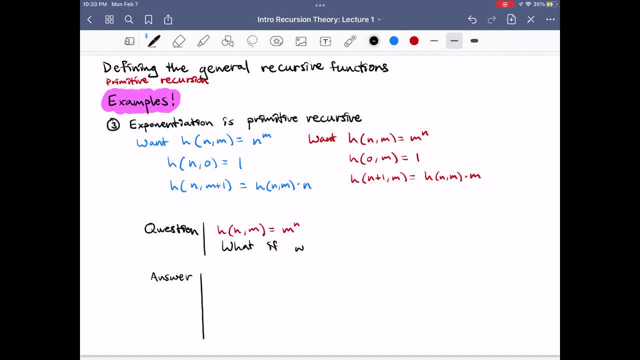 And what if we want the function that sends n comma m to n to the m instead? So in the right order. So is that also primitive recursive? It would be kind of troubling if it's not, because it's just a very simple modification of this one. 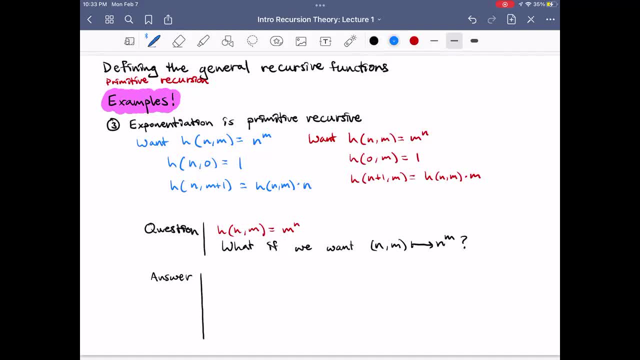 So the answer is we can just define a function by h composed with two projections: First the projection onto the second coordinate and second the projection onto the first coordinate. So this is the effect of swapping the input stage. So if we apply this to some inputs- n and m- 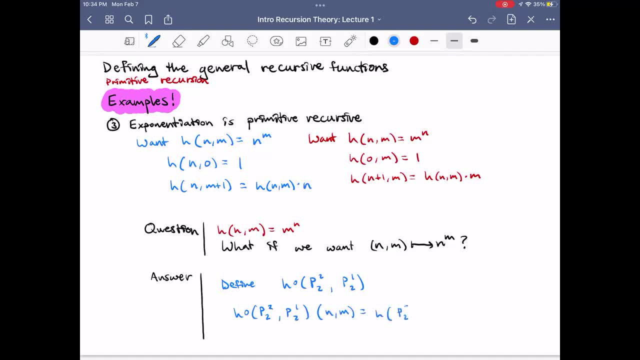 this is going to be h of p22 of nm and p21 of nm, So that's gonna give us m comma n, which we have seen is equal to n to the m. Okay, so sorry, I think it gets a bit confusing. 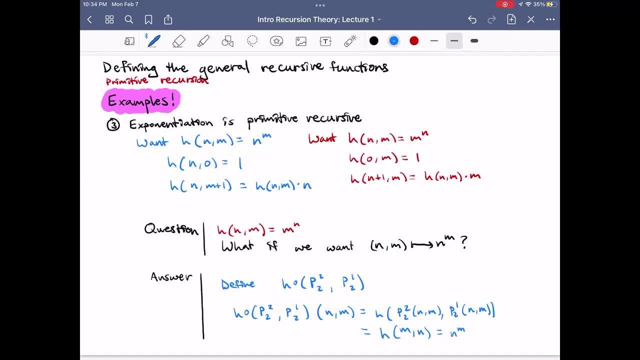 with all these little n's and m's and so on, but-. Okay, so sorry, I think it gets a bit confusing with all these little n's and m's and so on, but-. But the basic idea is, even though a primitive recursion, 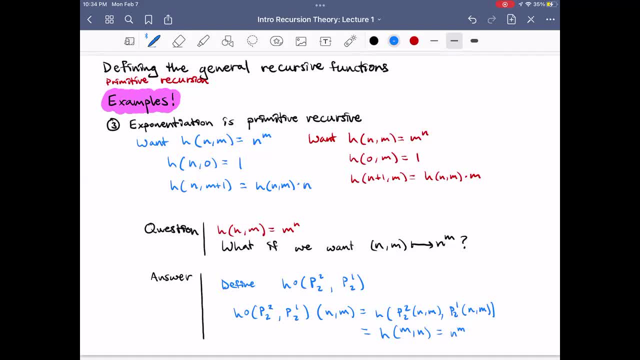 we had to sort of be doing recursion on one of the first input. in particular, it's easy to swap around inputs with these projection functions, So the primitive recursive functions are not super limited. Okay, and we'll do. maybe one last example a little bit faster. 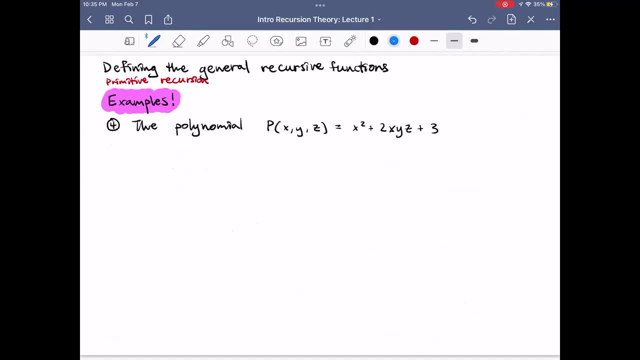 So say, we wanna show that this particular polynomial in three variables is primitive recursive. How can we do that? Well, basically, we can just compose a bunch of functions that we've already seen are primitive recursive. So let's define F1, and I'm going to refer to mult. 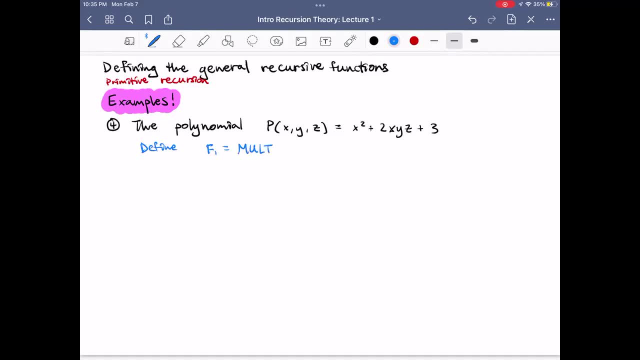 as the multiplication function that we've already shown as primitive recursive. Oops, sorry. What I want to say is mult of projection onto the first coordinate, together with projection onto the first coordinate. So our function is supposed to take three variables. The first one is X. 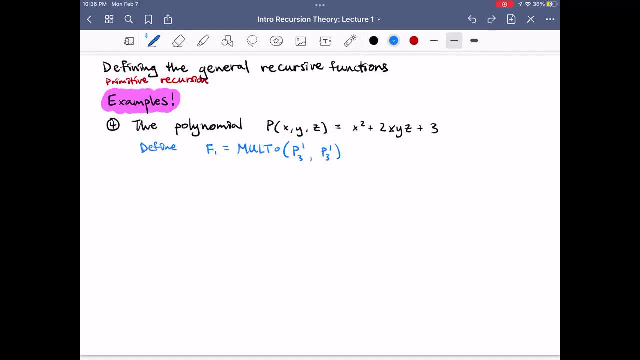 So this F1 is going to be X squared. I'll say it again in a moment. We can define F2.. We can try to get the function to X. So to do that we can take the composition of mult with the constant function two and P31 and so on. 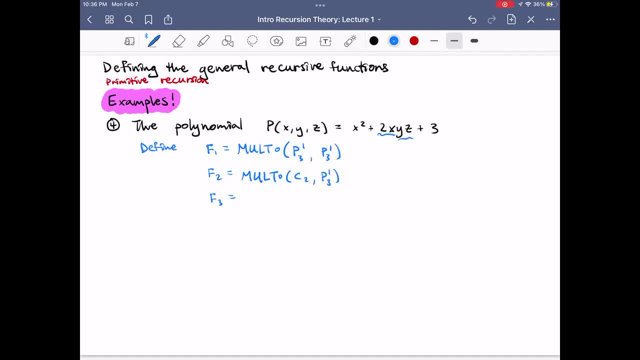 We can just kind of build up different parts of this expression. Oops, sorry, I made another mistake. So this should be F2 and F3, because now we want to multiply together these two terms And then we can add together this X squared term. 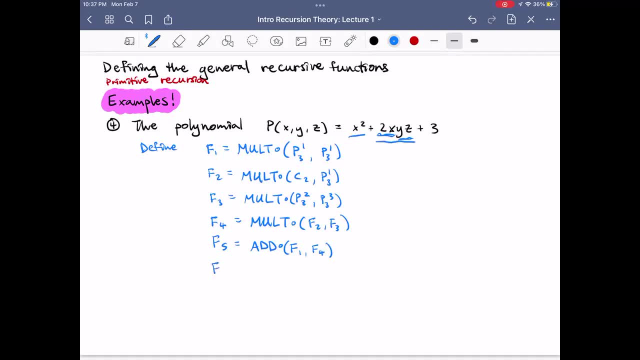 that we already have with this term, And then, finally, we can add together all that with the constant function three. So just to verify this: F1 of X, Y, Z, we're going to projection, so we're going to do this. 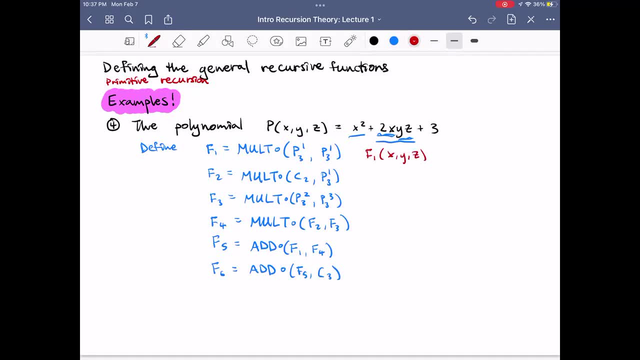 So we're going to take projection of the first coordinate two times and then multiply those two together. So this is going to be X times X, In other words X squared, and so on. F2 of X, Y, Z, we take the constant function two. 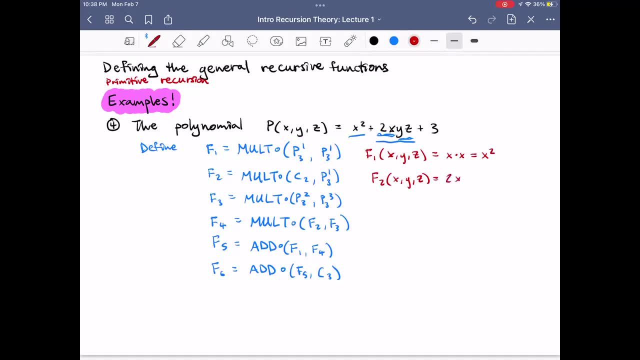 and multiply it by projection of the first coordinate, So it's two X. Here we take projection of the second and third coordinates and multiply them together, so we'll get Y, Z and so on, And then finally we can add together these two terms. 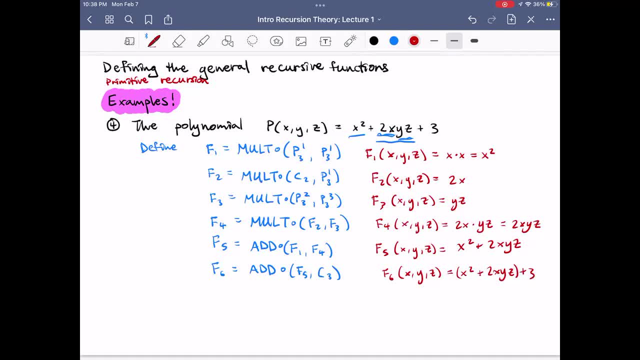 Okay, and we finally built up to the original polynomial And, in general, this is how you can show that things are primitive. recursive is you just keep building up more and more complicated functions And to get the next most complicated one, you either use composition or primitive recursion. 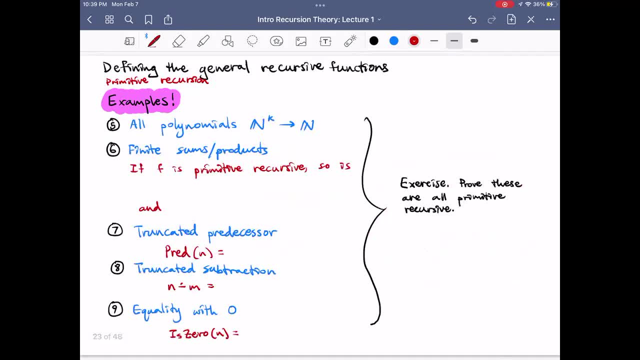 There's a lot more fun in this part And I'm sure that you'll find your answer very interesting. There's a lot more functions that you can show are primitive recursive, So here's some more examples. Every polynomial you can show is primitive recursive. 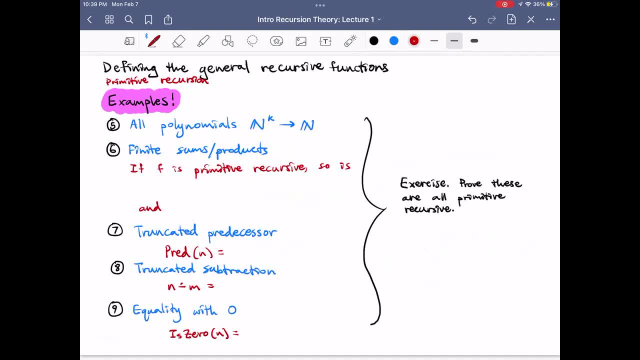 Also finite sums and products. So if f is a primitive recursive function, then so is the function that maps n to the sum of the first n values of f, As well as the function that maps n to the product of the first n values of f. 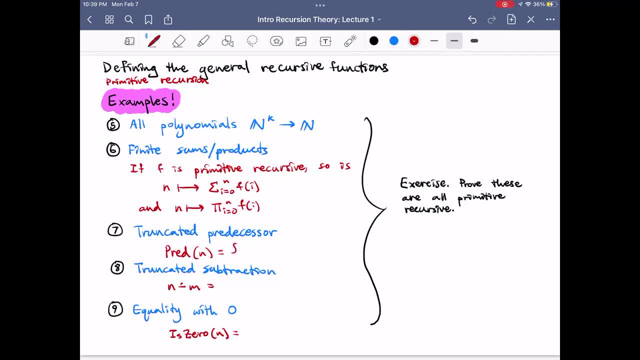 So those functions are primitive, recursive. The predecessor function, which subtracts one from a number unless the number is already zero and does nothing, This truncated subtraction. So this is a function that tries to subtract m from n unless n is smaller than m. 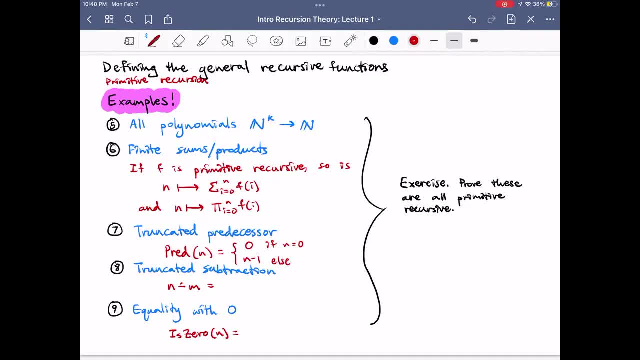 because then we would get a negative number that our co-domain is supposed to be the natural numbers. So then it just gives you zero. So this is the function: zero if m is greater than n and n minus m otherwise. So here we're just dealing with a quirk. 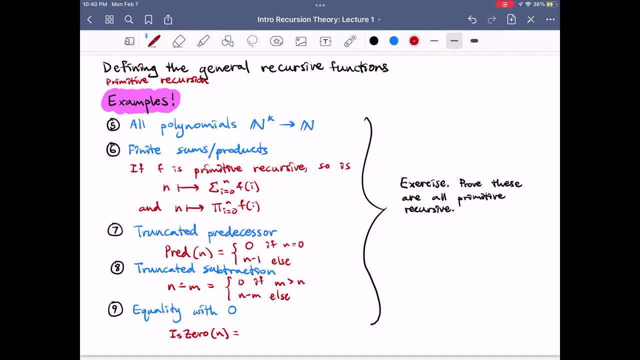 of the facts that we chose to look at functions from natural numbers to natural numbers. You might more naturally want to define subtraction as a function onto the integers, but we just said, for concreteness, we're only gonna use natural numbers, so we can't do that. 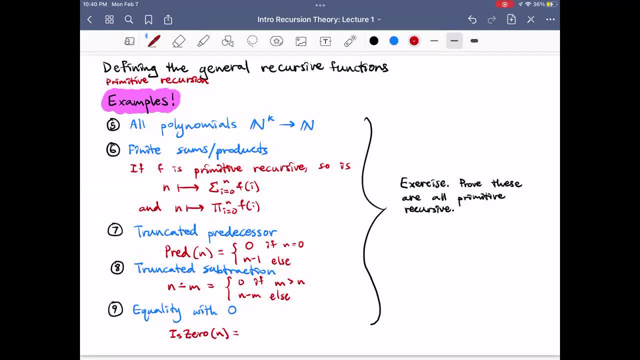 So you have to do some trick like this. And finally, the function checking if n is equal to zero. So let's say the function that's one if n equals zero and zero otherwise. So using just the kind of things we've done so far. 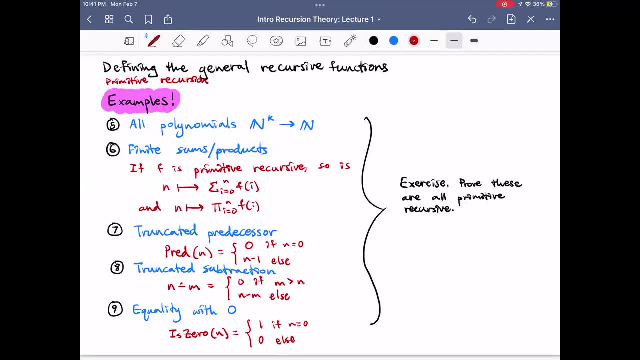 you can check that all of these are, in fact, primitive recursive. It's if you really want to understand how to define things by primitive recursion. some of these are maybe good exercises to do Next day. there's something else I need to say. 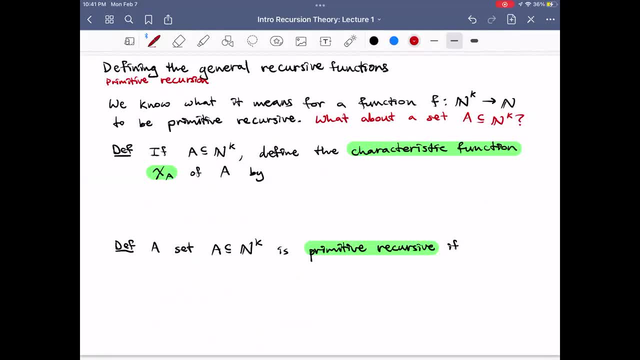 which is so far. we've just been talking about what it means for a function from natural numbers to natural numbers to be primitive recursive, And later we're gonna talk about what it means for such a function to be general recursive and so on. But what about a set of natural numbers? 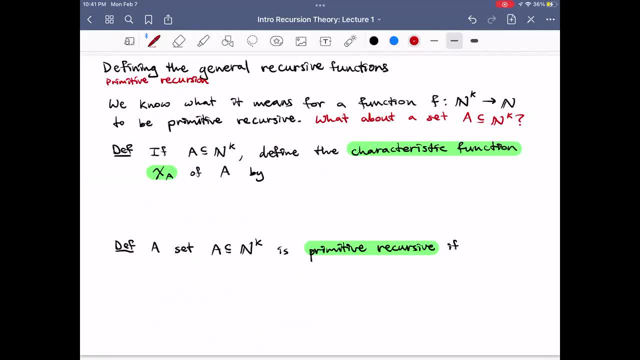 What if we want to say a set is computable? So we're going to define that just in terms of functions on natural numbers. So first let's recall definition. If a is a subset of natural numbers or some product of natural numbers times natural numbers, 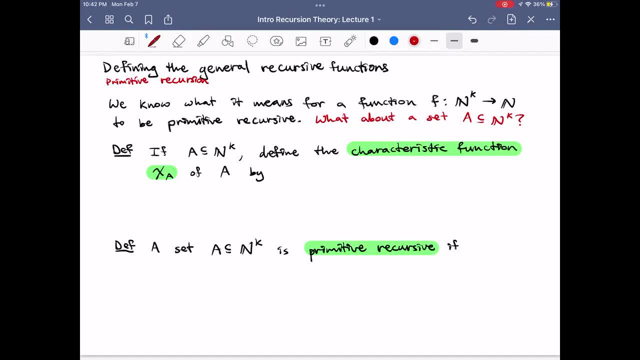 or whatever we'll define the characteristic function of a as the function. it takes K inputs in the natural numbers And it gives you zero if those K inputs are not an element of A And one if they are an element of A. So it just tells you whether the input it's given. 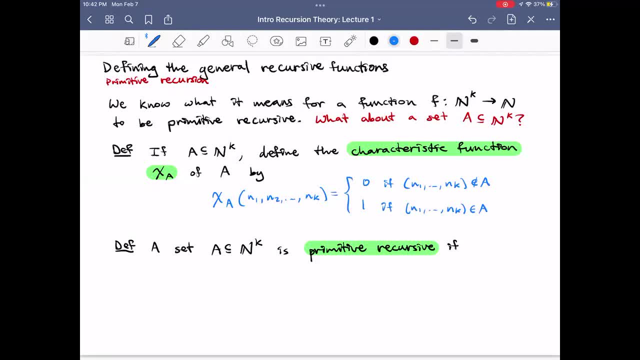 is an element of A or not. That's the characteristic function of a set, And we'll say that a set is primitive recursive if it's characteristic function is primitive recursive. Okay, so that's what I mean by saying a set is primitive recursive. 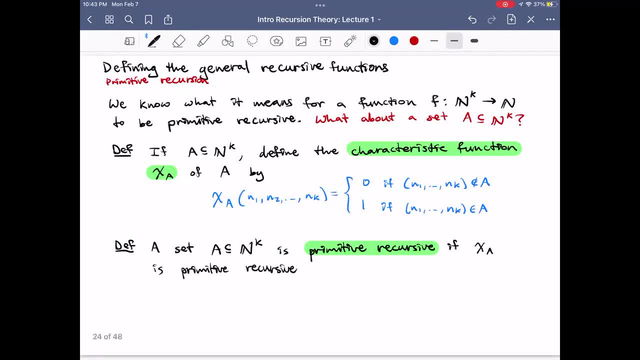 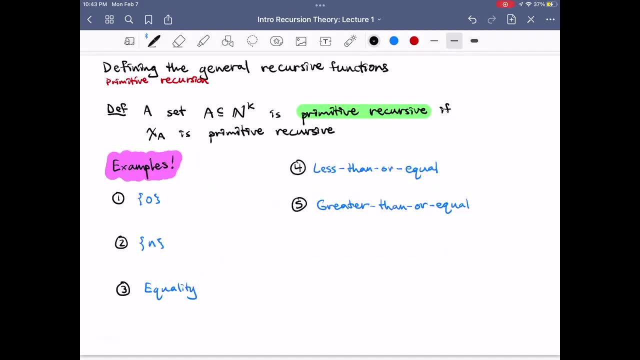 even though I said I would only talk about functions, And so let's see some examples of this. what kind of sets are primitive recursive? or at least a few. So first, the set that just contains zero is primitive recursive. That's because it's indicator function. 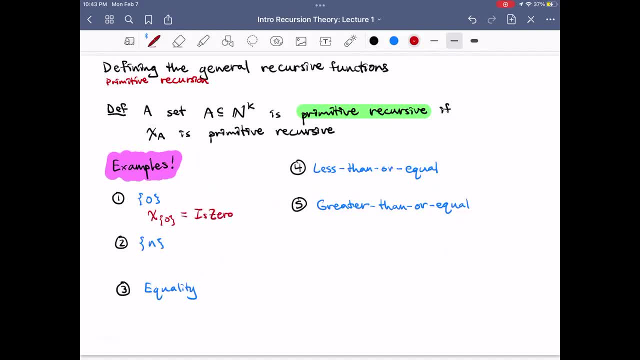 is just. this is zero function that I mentioned before. So if you do that exercise, you'll show that is zero is primitive recursive, which will show that this set is primitive recursive. In fact, For any natural number n, the set that just contains n is also primitive recursive. 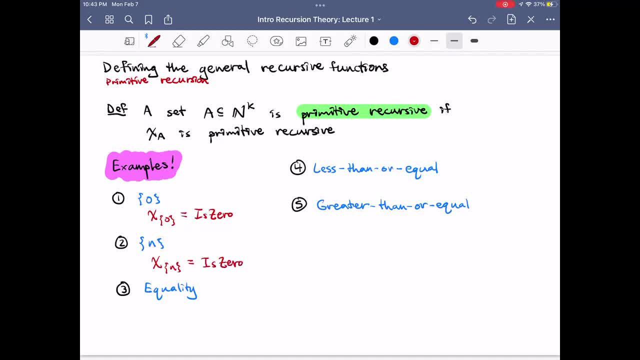 That's because you can define it as the is zero function composed- well, I need to maybe give this an input- composed with truncated subtraction of n minus m plus truncated subtraction of m minus n. So if n is not equal to m, then at least one of those will be a positive number. 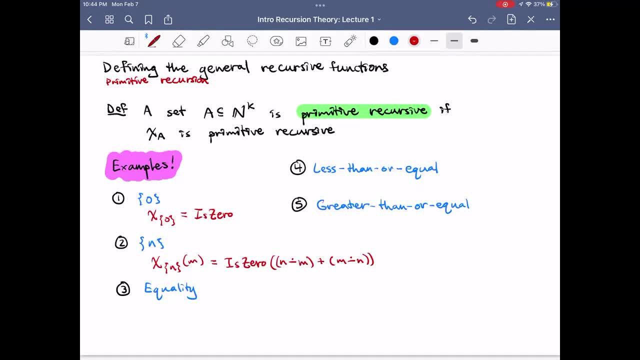 So their sum will be a positive number, So the whole thing will not be equal to zero. The equality predicate is also primitive, recursive. So this is formally the set n comma n, such that n is a natural number And this is of course a subset of natural number squared. 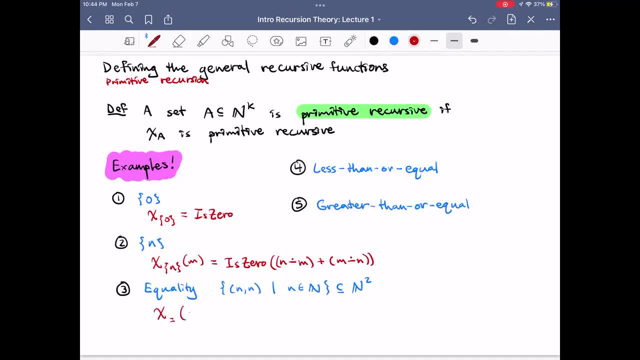 So that one the proof is almost identical. Its indicator function is simply is zero of n minus m plus m minus m, And the difference is: before, here this n was really the- you'd have to use the constant function with value n, and here you're using 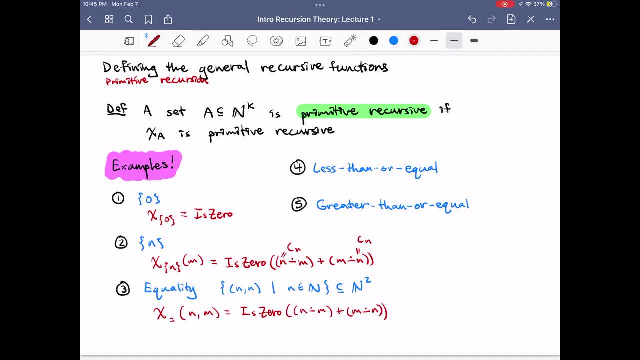 the input. Similarly, the less than or equal to and greater than or equal to function. sorry, sets are primitive recursive. So less than or equal to this is the set, Okay, Of n comma m in n squared such that n is less than or equal to m, And I guess you can. 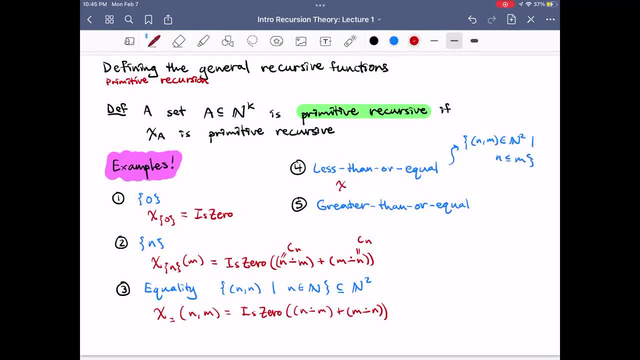 imagine what greater than or equal to set is And the indicator function of this this is equal to is zero of. in this case, it's just okay, Okay, Okay, So theilous. this is 2010,, right. 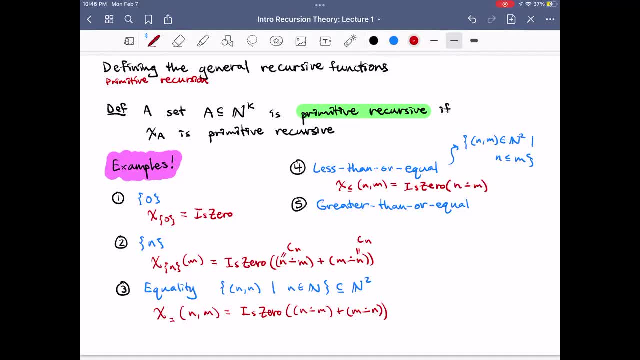 This is. this is the very same real, random function of exists today. Okay, Fu- Okay, And the greater or equal to is very similar, So one way you could define this actually is as the less than or equal to function composed with these two projections that swap the inputs. 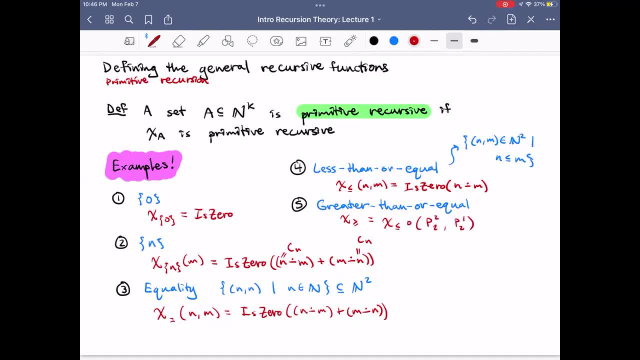 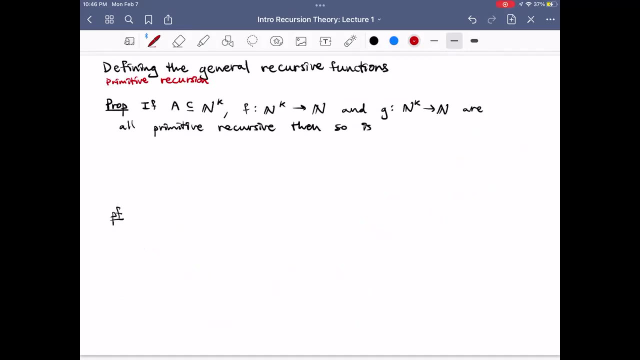 you could also define it directly. Okay, so if you believe that all these previous functions were primitive recursive, then all of these ones also are. And now here's maybe a couple of lemmas that tell you other sorts of functions you can define using primitive recursion. 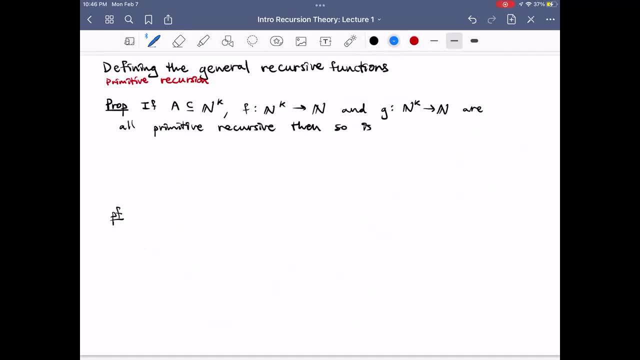 So suppose little f and little g are both primitive recursive and big A is a primitive recursive set, Then you can define a function using definition by cases on whether the input is an element of A. So then the function from n to the k to n. 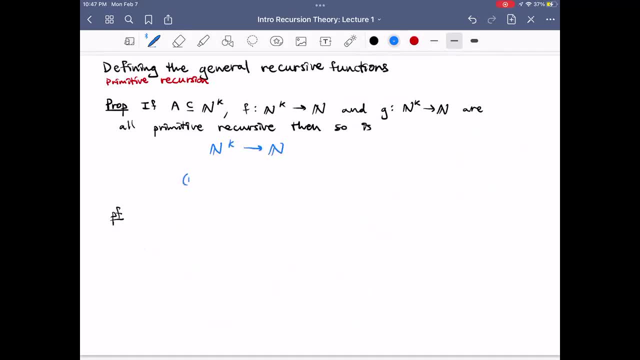 defined by it sends the input n1 through nk, It uses f. if the input is an element of A, It uses g otherwise. So defining a function this way is usually called definition by cases, And as long as the set and the functions you start out with, 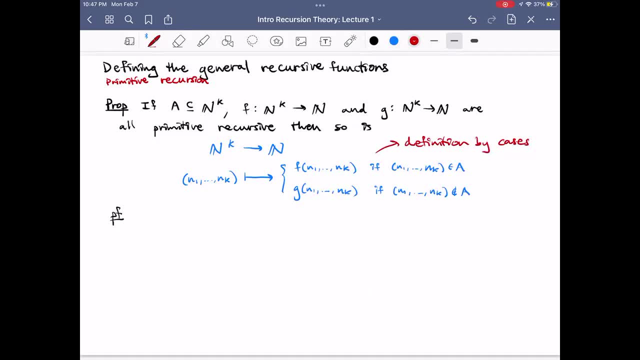 are primitive recursive. this is a primitive recursive set. This is also always primitive recursive, And I guess there's a few ways to do this, but one would be to note that this function is equal to indicator function of A multiplied by the function f plus one, minus the indicator function. 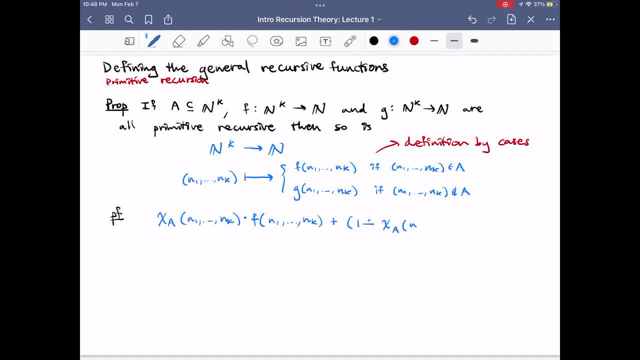 of A multiplied by g. So the indicator one minus the indicator function is zero if the input, if the input is equal to zero, if the input is equal to zero, if the input is equal to zero is an element of A and one if it's not an element of A. 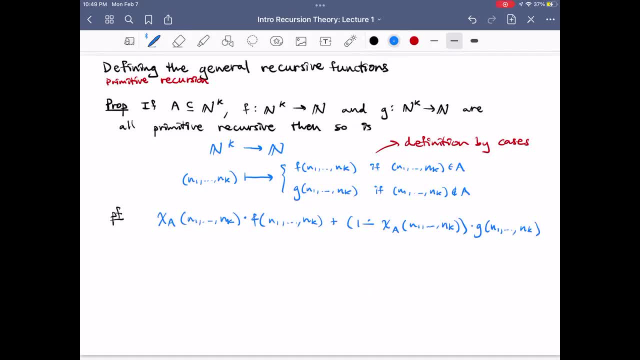 So you can then verify that this function is the function we want. So when you're defining things by, if you're trying to show that something is primitive, recursive, then you're justified in using definition by cases. Let's do another similar example to this. 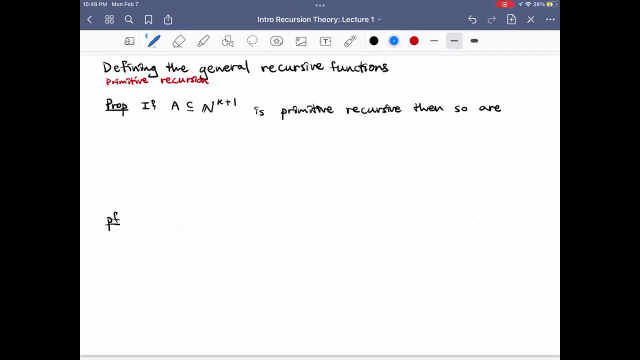 This is something called bounded quantification. So if A is a primitive recursive function, let's say if A is a primitive recursive set, then so are the two sets. I'm gonna call the first one. there exists X. less than or equal to n applied to A. 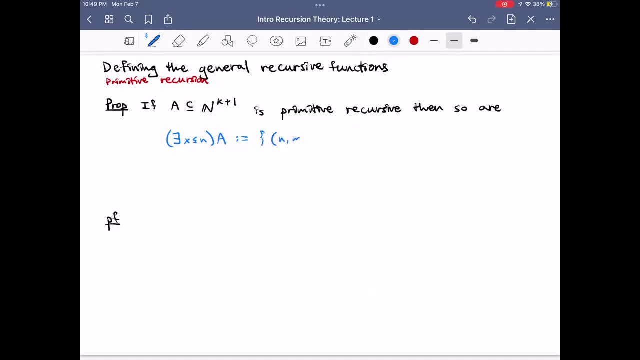 This is the set of n comma m, one through mk, such that there exists some X less than or equal to N, so that X comma M1 through MK is an element of A And similarly bounded quantification, the universal quantifier. 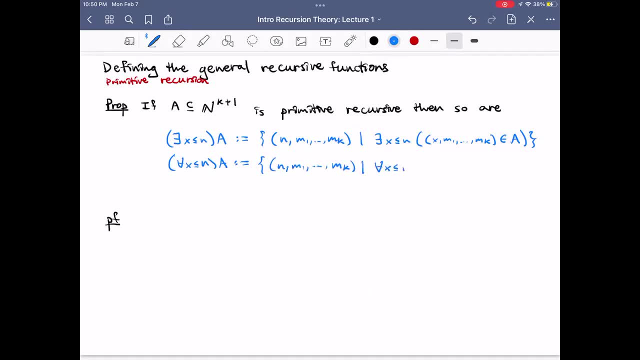 So these are both primitive recursive sets. These are both also subsets of N to the K plus one, And again this is called bounded quantification, And the proof is basically for the first one, it's indicator function. One way you can write it is as this: 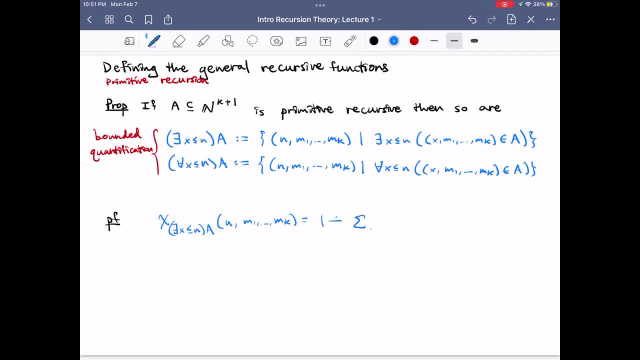 You want to draw an integer, then set your null, then get rid of the null And by doing that you can see that the first one is an open-structured set of N plus one. It's like a set of N minus one. 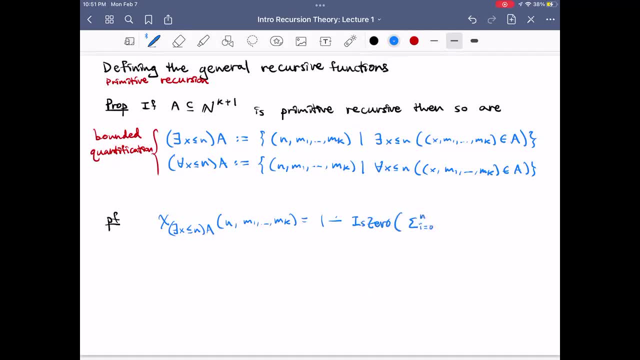 So you want to have that long, but not too long. It needs to be pretty easy to get that long. but it's just a study to get the small, but it's not very difficult to get that long. So you wanna have the long statements. 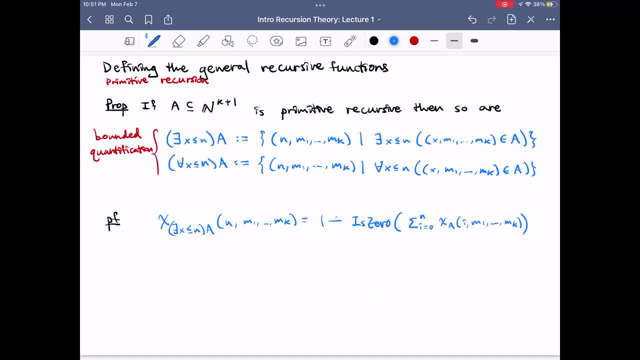 So if there doesn't exist such a little x, then that sum will just be zero, And if there does exist such an x, then the sum will be non-zero, And when you take one minus it, you'll get the right thing. 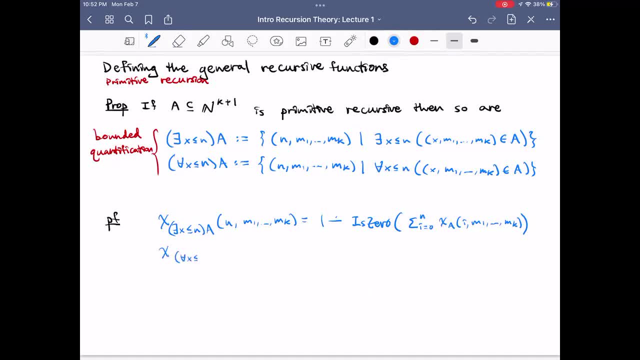 You can do something very similar for universal quantifiers. So yeah, I mean, this is the kind of thing maybe where it's easier to just work out on your own why this works than it is to hear somebody explain it. And I guess the point of all this is that we can build up a lot of functions that are 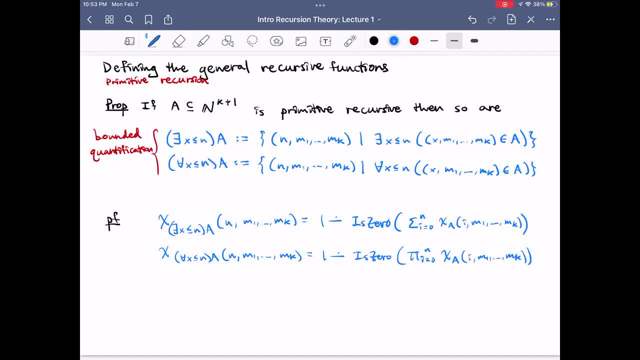 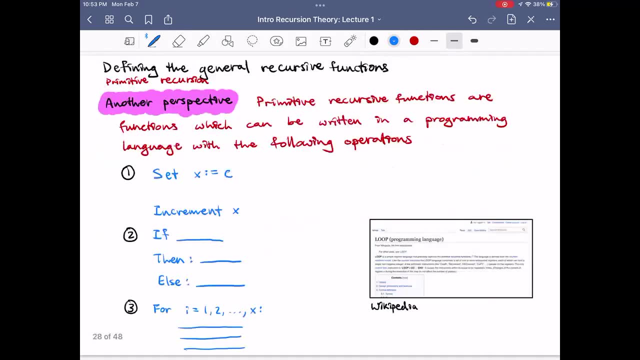 prone to recursive. We can build up a lot of tools for building up more functions. So, yeah, Yeah, So primitive recursive functions actually have a lot of closure properties. I want to maybe not do more examples of that, but mention some other perspectives about. 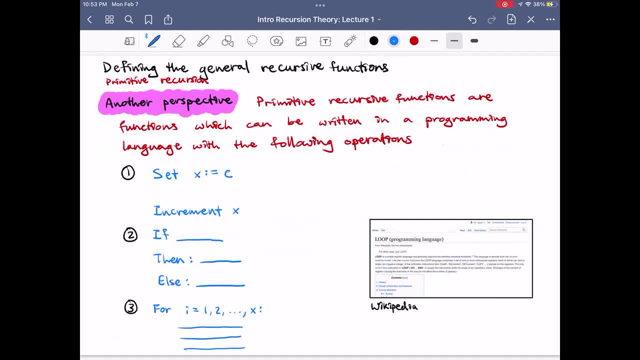 primitive recursive functions, And then maybe we'll take a little break and then we can move on to actually defining computable functions. So one perspective is that another way to define primitive recursive functions is to specify some programming language. So this is a programming language where. what can you do? 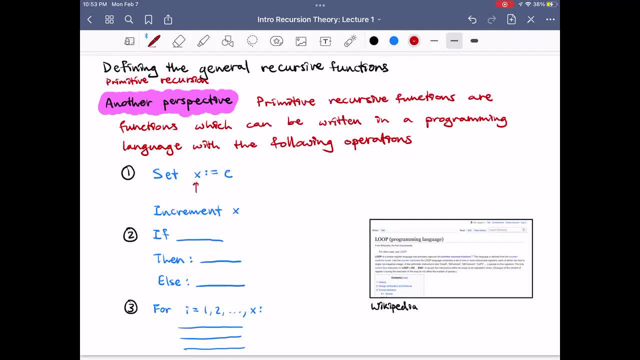 You can set a variable equal to some constant. So here X is a variable and C is some actual natural number. You can increment any variable, So you can add one to it. You can have if-then-else structures And the things you're allowed to put in there. 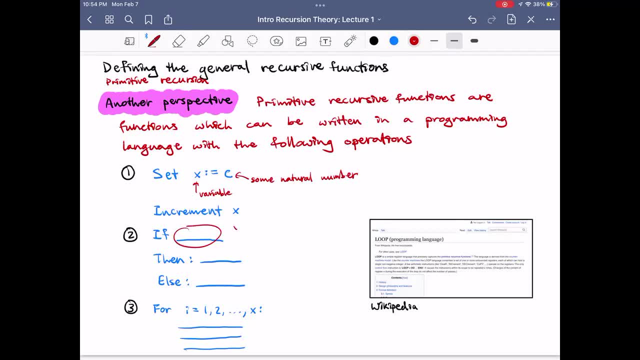 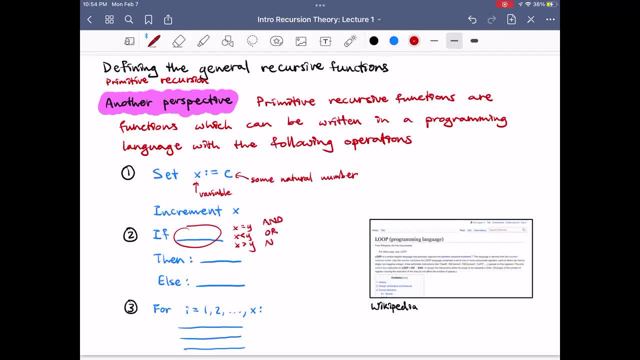 less than Y, X is greater than Y And you're also allowed to combine them with ANDs and ORs and NOTs And finally, you're allowed to have four loops. So if X is a variable, you can loop from I equals 1 to X and do something in the body. 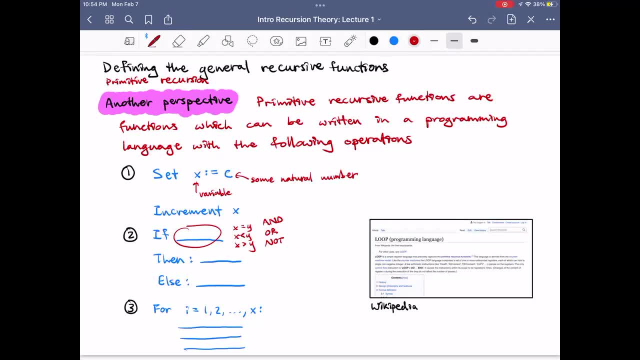 of the loop. So if you have a programming language with basically this instruction set, then the programs you can compute with that programming language are pretty much exactly the primitive recursive, are exactly the primitive recursive functions And you should think this, for loop corresponds to primitive recursion. 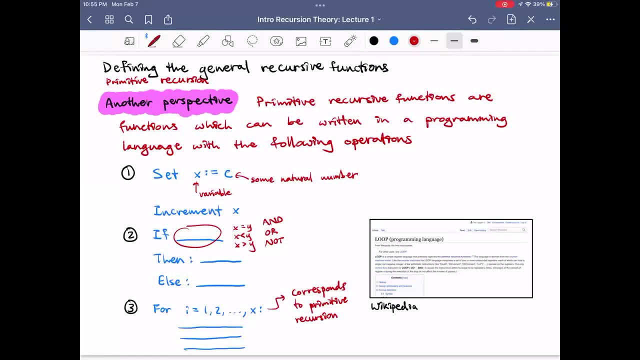 So, in primitive recursion recall, if you wanna know what is the value of like H of N plus H of N, well, you can figure out H of N in terms of H of N minus one, which you can figure out in terms of H of N minus two. 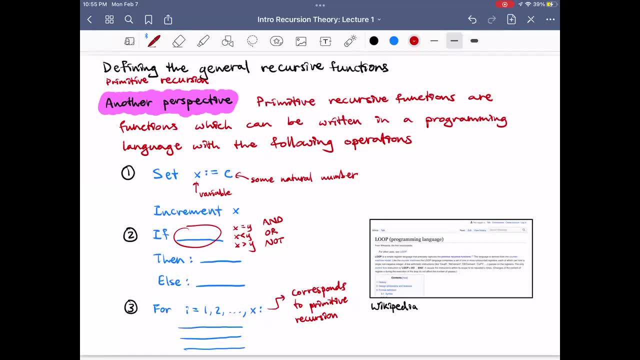 and so on. So that corresponds to some kind of for loop where you build up from H of zero, H of one, H of two, all the way through H of N, but you only need to do N steps. You don't need to do like some much larger number of steps. 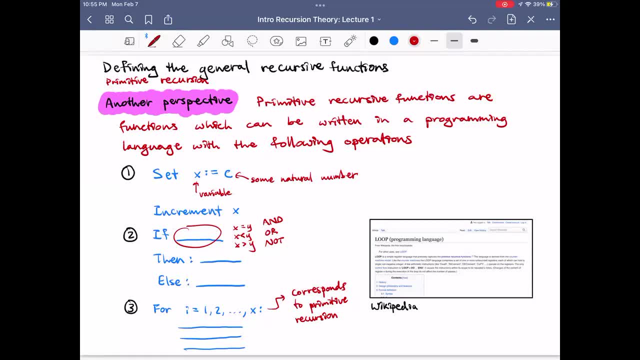 to figure out H of N. So basically, one way to think of primitive recursion is that it corresponds to for loops, And what makes this programming language weaker than other programming languages is it sort of only has for loops and no while loops. So if you're not familiar with programming, 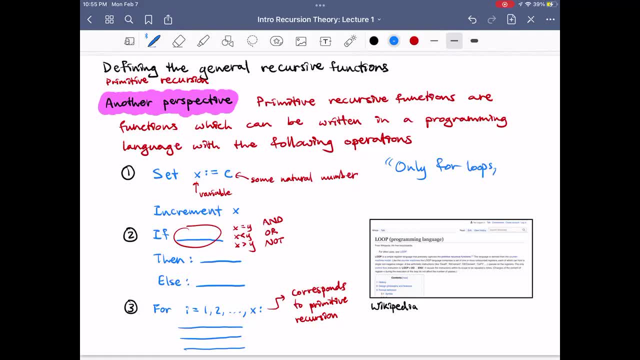 you can maybe ignore this perspective and the other definition we gave is perfectly valid, But this is maybe useful way to think about it And there is even like a formal version of this. So, for instance, there's a thing called the loop programming language which is exactly like this. 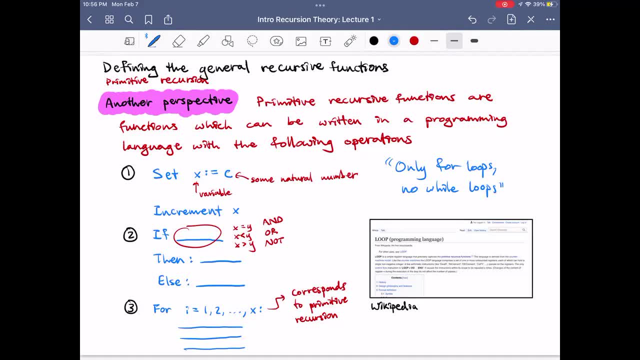 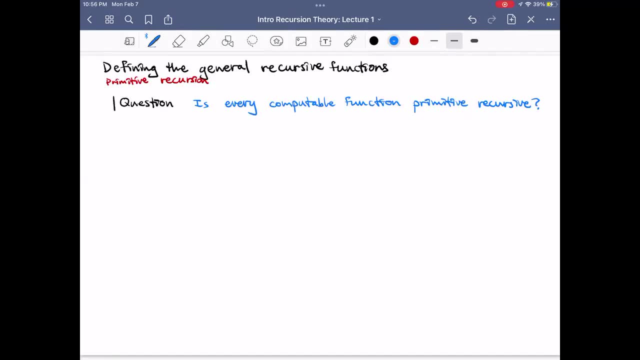 You can look it up if you want to. Okay, So let me know, I'll discuss one last thing and then maybe we can take a short break. So I kind of already said the answer to this, but one could ask, is every computable function. 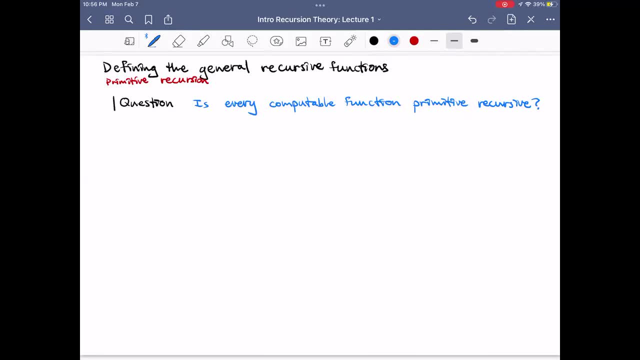 a primitive recursive. So there's some intuitive argument that every primitive recursive function is computable. but is a true the other way around? And actually it turns out the answer is no, and this was first proved by some guy named Wilhelm Ackerman. 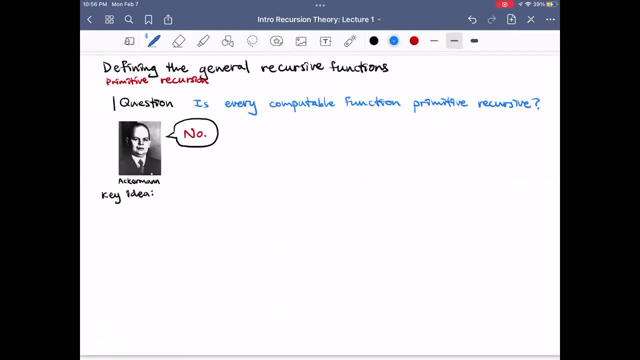 And this was actually approved before anyone gave a definition of computable function. So at the time maybe it wasn't obvious at first whether or not primitive recursive meant computable. And the key idea of the proof is basically that primitive recursive functions cannot grow too fast. So there's some. if f is primitive recursive, there's some limit on. 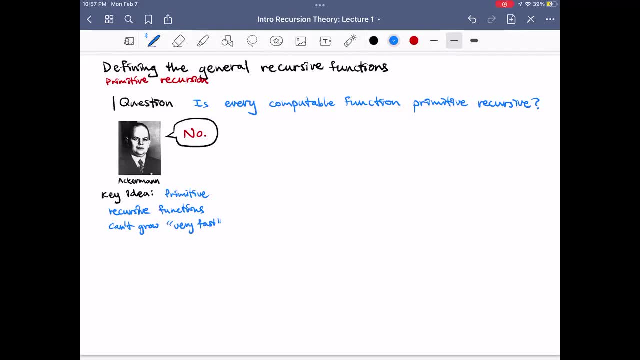 how big f of n can be in terms of n, But general computable functions can be larger. That's sort of the idea of the proof. That's a bit vague, So I want to maybe give some indication of how the proof works, but not actually give a complete. 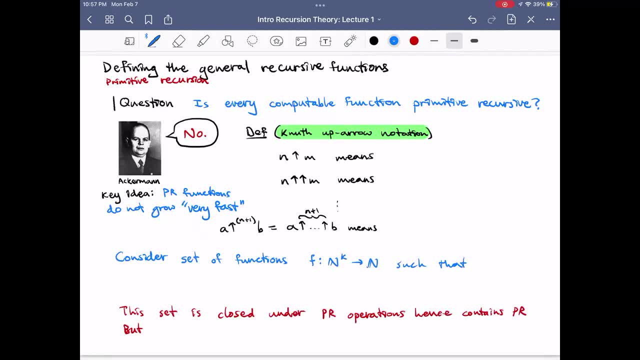 proof. So one way to describe it is in terms of this thing called newth up arrow notation, which is some way of describing large numbers. basically So n up arrow m, this means n to the m. So one up arrow is exponentiation, And each additional up arrow you add. 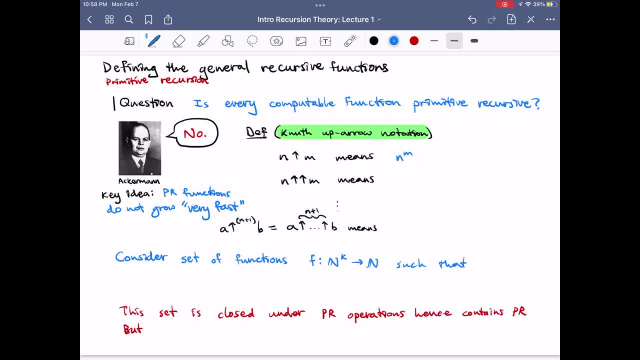 you repeat the previous operation, m times. So n up, arrow, up, arrow m means you take n to the n and then you take that to the n. Well, I should really be putting the n's down below, But anyways, you have a tower of exponents of length, m, So you iterate exponentiation, m times And so on. So in particular, if you have m times, you have a tower of exponents of length m, So you iterate exponentiation m times. But when you have m plus m up arrow, m, that's a, that's a new thing. So you write n plus one up arrows. 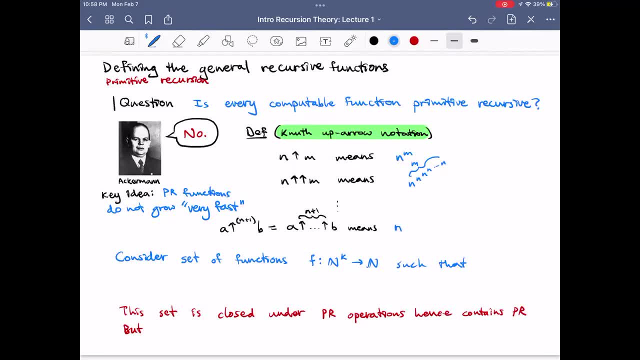 What does that mean? That means you start with n- the argument on the left- sorry, now I'm calling it a- apparently the argument on the left- And you write n up arrows And you apply that. maybe let me describe it sort of the other way around. So you start with a And you put n up arrows with a. 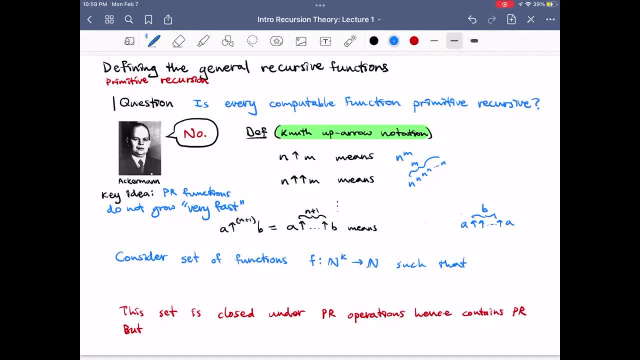 or I should say b up arrows with a, sorry. and then you take that and you do it again with n up arrows. uh, oops, sorry, I've made two typos now, so, uh, let me, let me restart. so what does it mean to do a n plus one up arrows b? it means you start with a and do n up arrows of a, and then you repeat that. 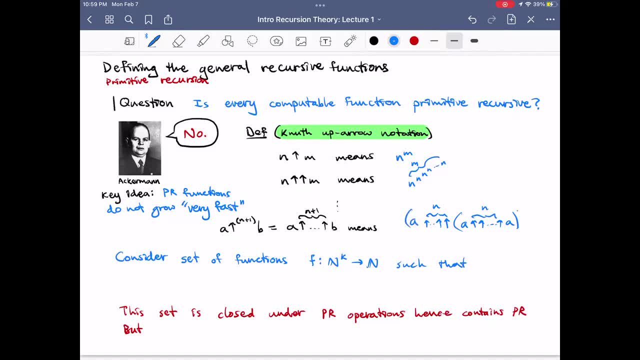 again. so you do n more up arrows of a and then you keep repeating that and the number of times you repeat it is b? um. so each, each time you do some set of up arrows, you're doing n of them. so, as I said, you start with exponentiation. the next level is, like you, iterate exponentiation. 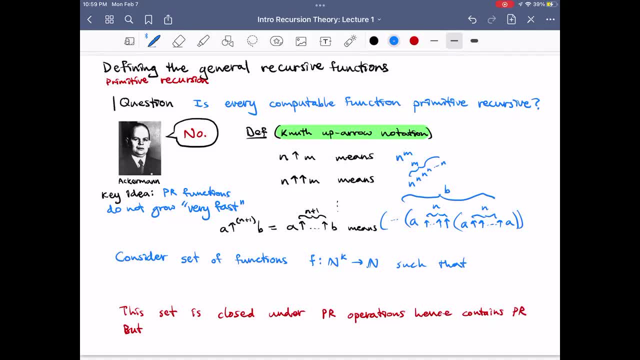 m times. the next level is you iterate that m times. so this is some sequence of very fast growing functions, um, um, um. and it turns out that, like every primitive recursive function is bounded by one of these. uh, so if we consider the function set of functions f, from n to the k to n, such that 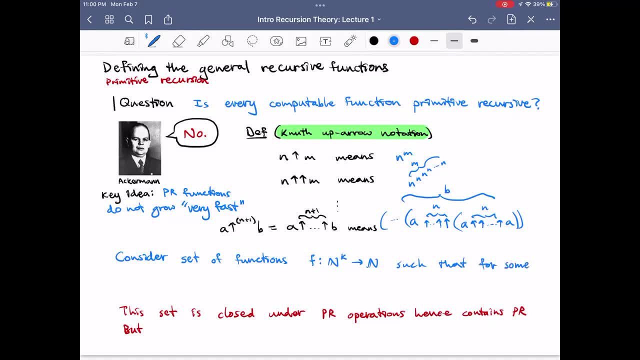 uh, for some uh, n? um. f is eventually always less than or equal to n. f is eventually always less than or equal to uh. it's eventually bounded by um n1 plus n2 plus so on. uh, and then n up arrows of again n1 plus n2 plus so on. 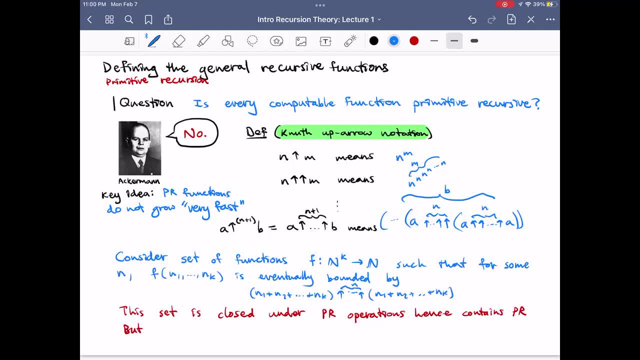 and then n up arrows of again n1 plus n2 plus so on, uh, and then n up arrows of again n1 plus n2 plus so on. um, it turns out that set of functions is closed under the primitive recursive operations and hence it contains all the primitive recursive functions, so functions whose growth rate is bounded by some. 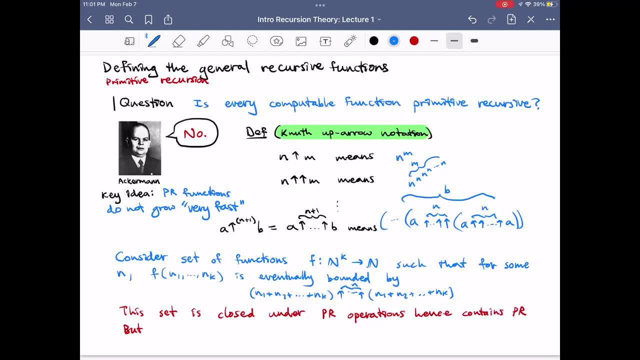 number of newth up arrows. those functions are all contain all the primitive recursive functions. so this is what I mean when I said the primitive recursive functions can't grow that fast, they can't grow faster than some finite number of up arrows. but but the function which takes n as input and gives you as output n, with n up arrows, n. 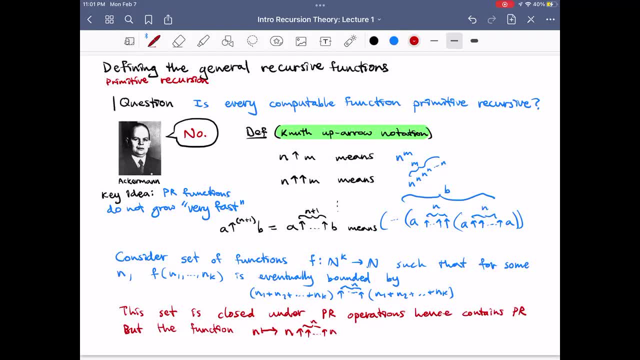 So this grows faster than any finite number of up arrows And if you believe what I've said, that means it's not primitive, recursive, But it is computable. I've kind of actually just described to you how you could compute it with my definition of the up arrow notation. So the whole idea of the proof basically, is to find 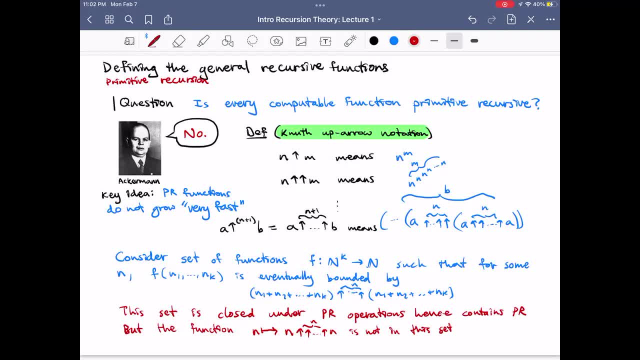 some set of functions and show that every primitive recursive function is bounded by one of those functions, and then construct a computable function that grows faster than all of them. So that's the idea of the proof. Now we'll talk about how to expand the definition. of primitive recursive to actually capture all of them. So let's get started. So I'm going to ask you to start with the proof And I'm going to ask you to start with the proof. So let's take a few minutes break. So I'm going to ask you to start with the proof.